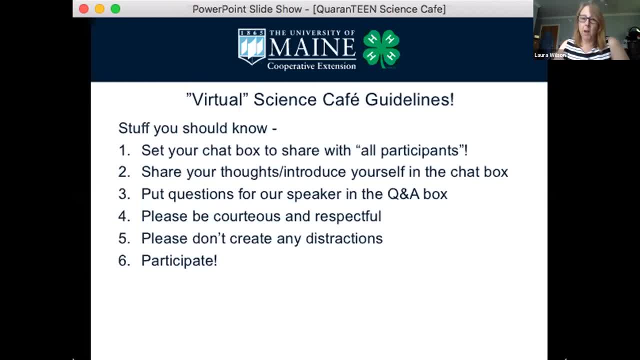 of the University of Maine brought to you by the University of Maine Cooperative Extension. I hope you all take a second to introduce yourself in the chat box. Please just share your name and your town if you would. That would be fantastic. Here at Maine 4-H we have Alice Philbrook monitoring the chat And Jesse Brainerd is hosting our Q&A today. 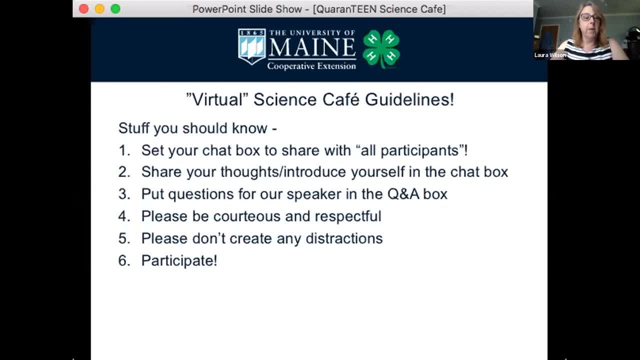 Also working behind the scenes. I'll be helping out so that all of this runs smoothly. We're going to keep this session simple. today, Our guest will share some of her cool research and a bit about herself. She's got some really cool photos to share with us today, And then we'll have plenty of time for you to ask questions. 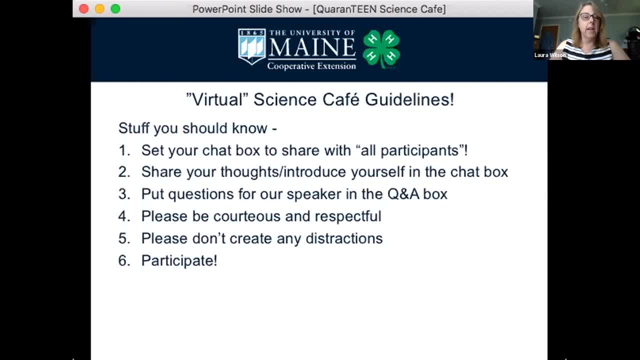 We'll use the Q&A box at the bottom of your screen to get questions to her. Quick note about the chat. We'd love to see your reactions to what our guest presents, But please keep on topic in the chat and we'll be able to keep chat open for you today. 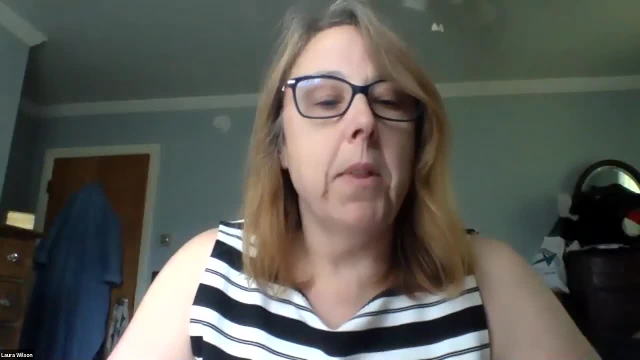 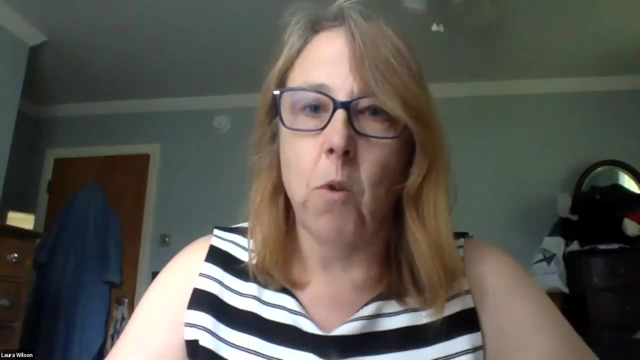 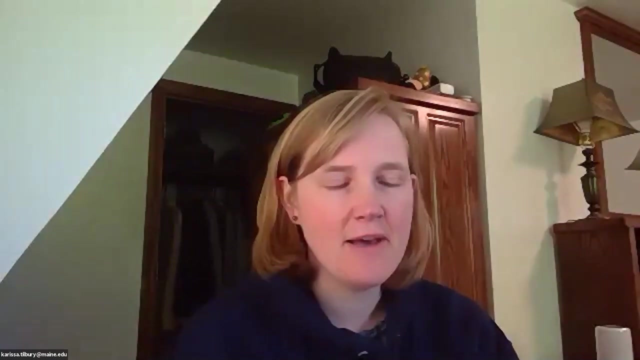 So it's my pleasure to introduce Dr Carissa Tilbury. Dr Tilbury, would you please tell our participants about yourself and your work? Absolutely So, I'm Dr Carissa Tilbury. I'm an assistant professor at the University of Maine. I have been in Maine for almost four years. 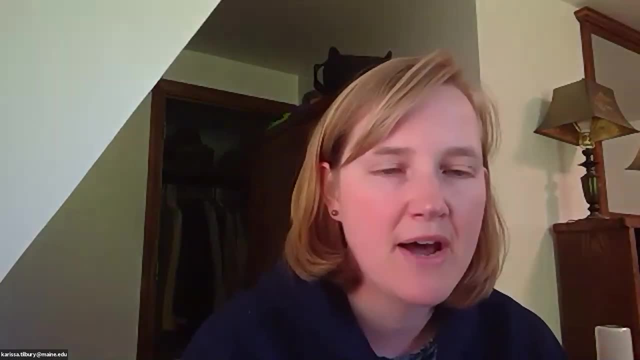 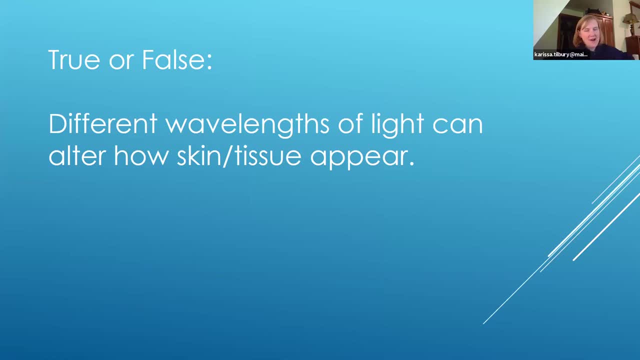 from the University of Wisconsin-Lincoln And then before that, I got my PhD. awesome, you guys are brilliant, absolutely so. you saw that on the previous slide, so that's why, you know, maybe at Christmas time, when you take that nice Christmas photo, you find the perfect light. 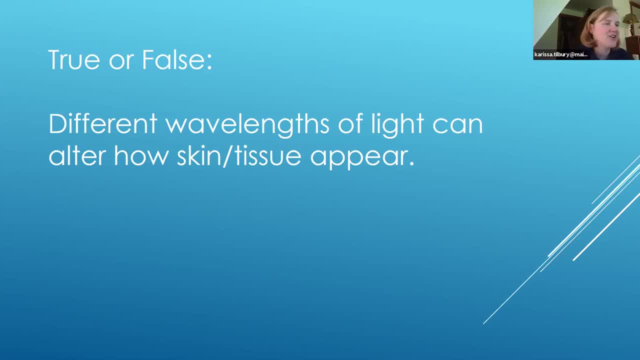 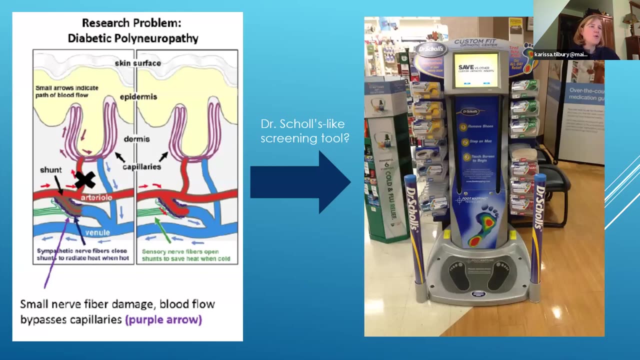 bulb that's going to make your skin appear the most blemish free. all right. so what can we do with that different information about light? so one particular problem that I'm working on in my research group is trying to understand diabetes, and particularly a disease that comes as a result. 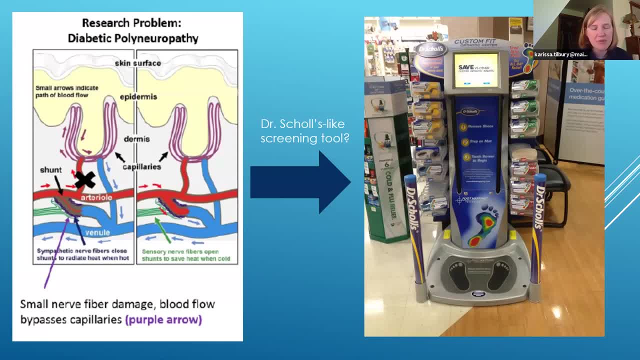 of being diabetic, so I'm assuming that most of you probably know someone in their life that suffers from diabetes and might have to prick themselves and take their blood glucose levels every day. so why people need to do that is they need to make sure that the rest of their body is. 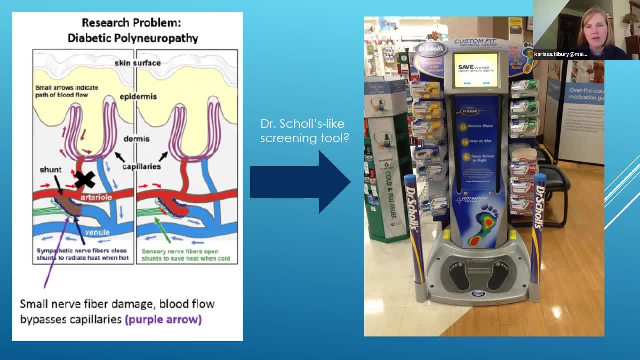 going to maintain proper nutritive flow and keep those tissues alive and well you. so. one of the common things that happens to diabetics is they have this disease called diabetic polyneuropathy. so basically what that means is that their nerves die back and then. 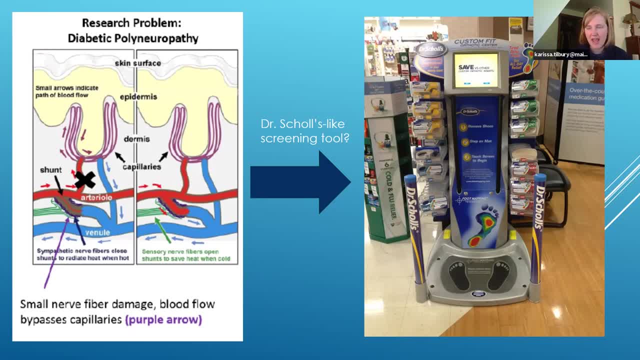 once their nerves die back, they can't feel the tissue, they can't maybe feel their toes and they also aren't going to be able to heal very well, and then they might end up with an amputation of their right toe or maybe, even worse, their foot. and that sounds very scary and it is. 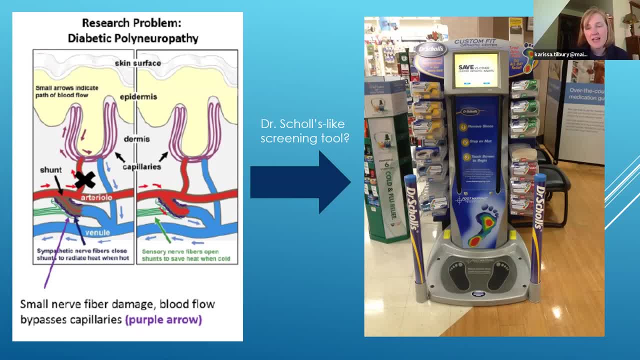 very scary and it's not going to be able to heal very well and then they might end up with an amputation of their right toe or maybe, even worse, their foot. and it's very dominant. it happens a lot, in fact. if you look across the entire world, someone is getting their foot amputated every 30 seconds. 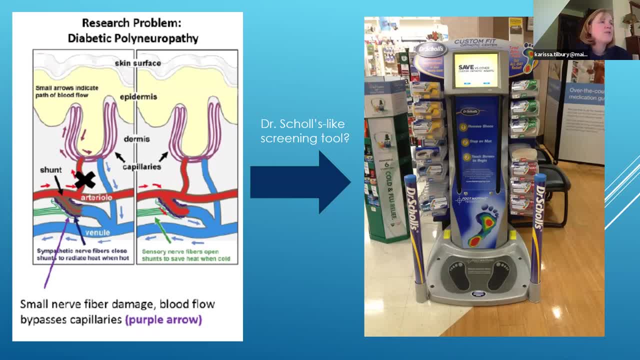 due to diabetic polyneuropathy, so the treatment and the diagnosis for it is really quite poor. so currently how you're diagnosed is literally a doctor touches your, your foot or your hands and asks with a filament, a little piece of plastic, and asks if you can feel it or not. so that's not very. 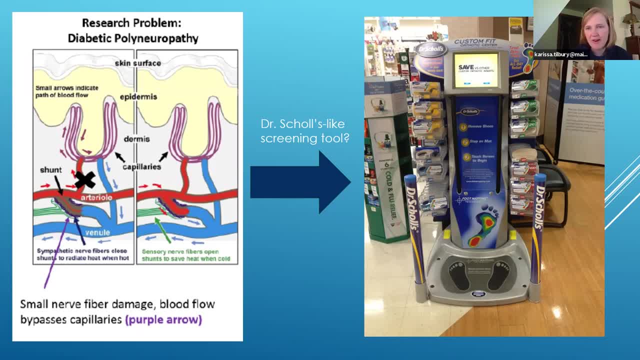 quantifiable. it's very subjective. you probably are anxious, you're thinking that you should be able to feel something, and maybe you're saying yes, even though you can't say anything. furthermore, by the time that you diagnose it, in that approach, the damage is so severe that we can't actually 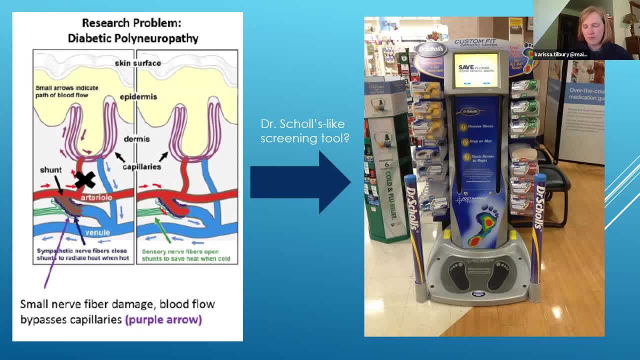 treat it. there's no way to prevent the the further loss of innervation or nerve or sensations that you have. so that led me to question like: could we detect this earlier, because i've seen lots of family members that have diabetes. so turns out that if you go and look at the pathology, 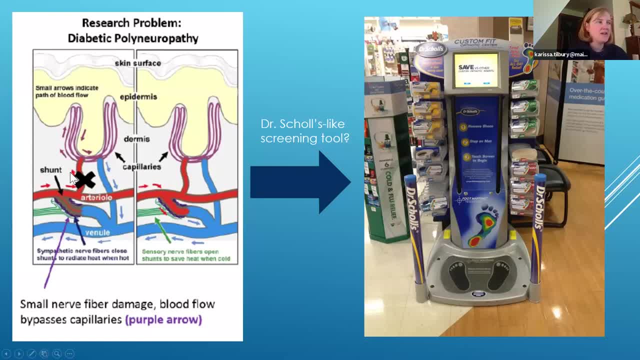 or the physio physiology of diabetic polyneuropathy. we see that we have these vessels in our bodies, so we have arterioles, which are just small blood vessels that are carrying oxygenated blood, and those arterioles are going to lead up into these structures that are shown here in these 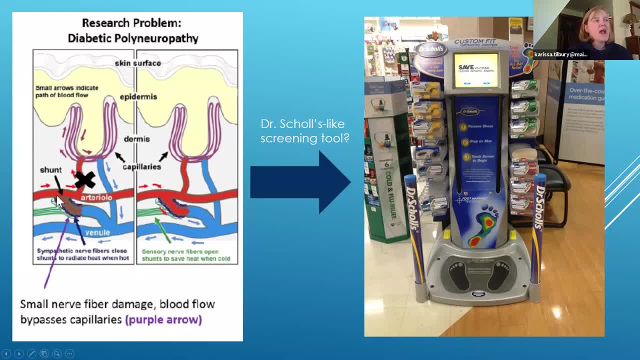 purple loops called capillaries, and those arterioles have little nerves that are innervating, causing these arterioles to pulsate back and forth, to have variation of diameters. and that variation of diameters, while doesn't seem to be that important, is dramatic and it changes the 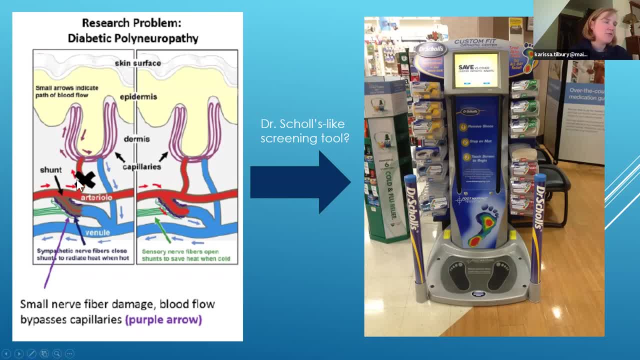 way in which the flow through the blood is going to go through. so in in diabetics they've seen that these nerves die back. and then what happens is these arterioles aren't able to change their size. and then what happens is the resistance to flow in those vessels becomes so great that they're not going to go up into these. 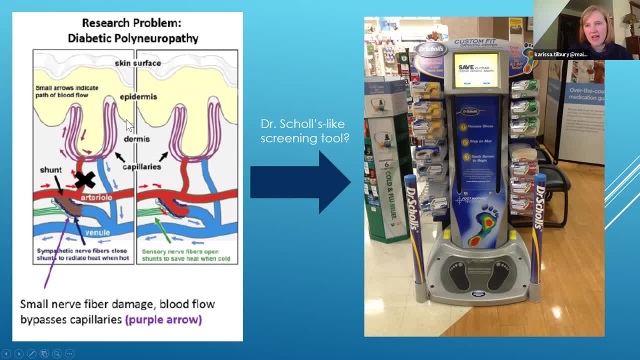 capillaries and deliver nutrients and exchange gases to those tissues. so, fun fact, if you're a cell and you're further away than 50 microns. so from a blood vessel, from one of these arterioles, you're not going to receive adequate nutrients. so 50 microns is really a very small distance. 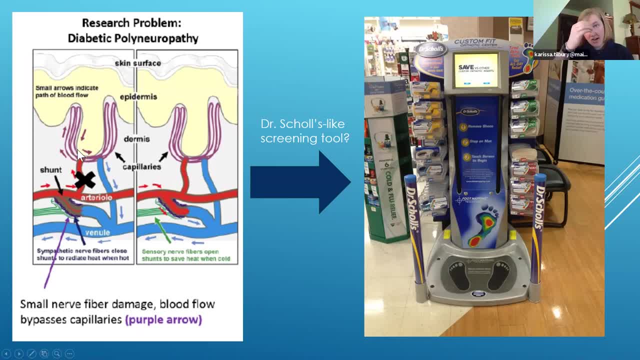 so if you look at a blood vessel from one of these arterioles, you're not going to receive adequate nutrients. but if you look at one strand of your hair, a single hair is about 100 microns, so think about half of a single strand of hair. you have to be that that close to a blood vessel supply in order. 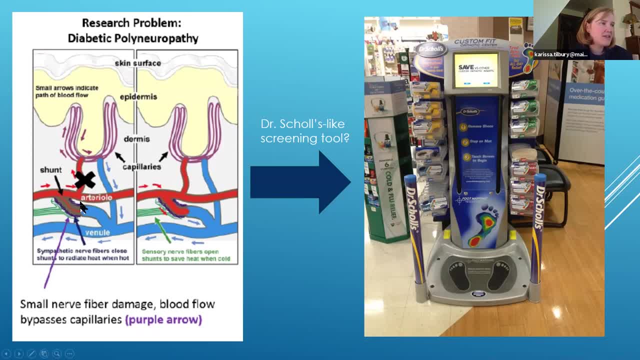 to sustain life. so in diabetic neuropathy, when we get these dieback and nerves, we're not. we're not going to get the flow up through these purple loops anymore. so you can imagine why wound healing is such a problem in diabetics. damage in the first place is a problem because 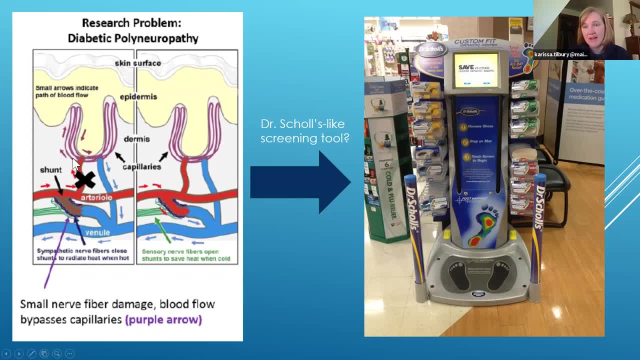 you're going to be a lot further than 50 microns away. those cells to maintain health, health aspects. so now i've described to you the physiology of diabetic polyneuropathy. so if we could detect it at that level, maybe we could actually treat it and prevent it from getting worse. so when you guys go, 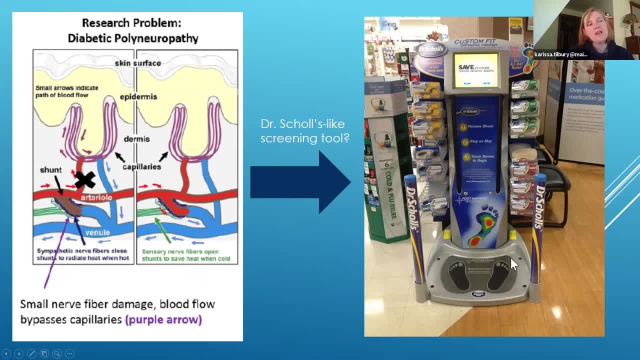 to walmart or walgreens or any other sort of big box retailer store. you probably have seen these artificials custom fit orthotic center. right, you stand on it and you get what, what size orthotic you should should wear. maybe you haven't done this, but maybe you've watched your parents do that. 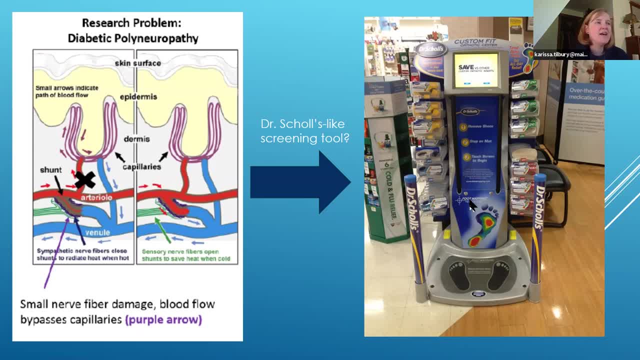 so a kind of crazy out of the box idea is that, instead of having this sort of screening protocol that we have right now for diabetic polyneuropathy, what if, instead of selecting your, which insole you should use, what if, instead, we turn this machine? 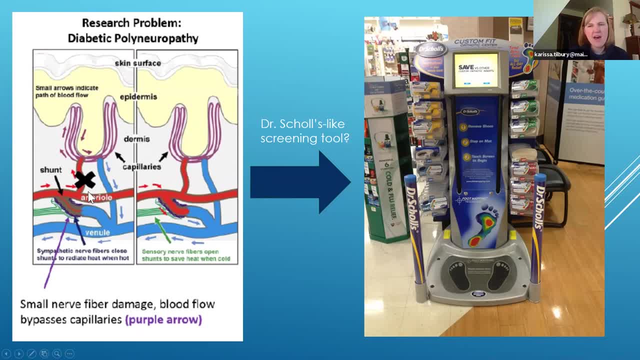 that's going to use light to try to understand how well are your nerves functioning and specifically how well are your nerves functioning around these arterioles. So that seems probably like a pretty crazy idea, but it's not as outlandish as you might think. 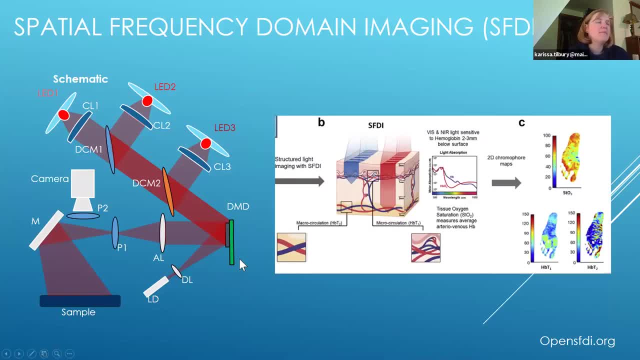 So enter in spatial frequency domain imaging. So this is a schematic that you might have in inside the Dr Scholl's machine. So we have three LEDs here of different wavelengths, because we know that depending on what wavelength of light we use, we're going to see different things. It's going to encode various structures. 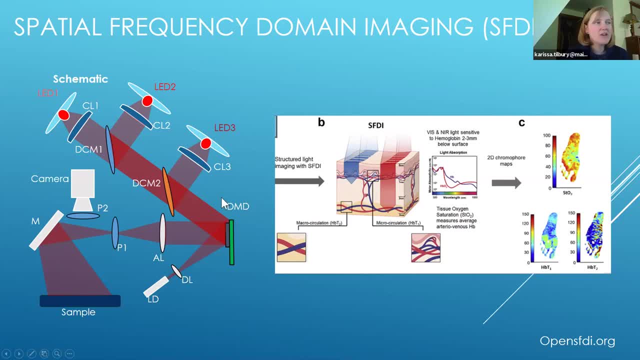 So we're going to have three of those, We're going to combine them all And then we're going to use this DMD here. So this stands for a digital micromirror device. So this isn't really anything fancy. This is the same thing. This: the three LEDs. 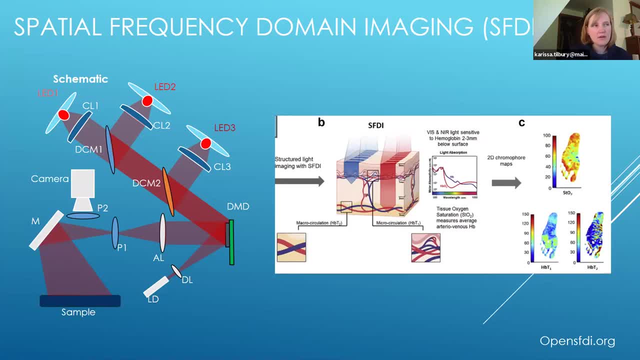 Oops, The three LEDs plus this DMD is effectively what is in every single projector you've ever used in your entire life. So, basically, I'm just recreating a projector And I'm going to project patterns of light onto a particular tissue So I can project that onto your face, I can project that onto your feet, I can project that onto your hand, wherever. 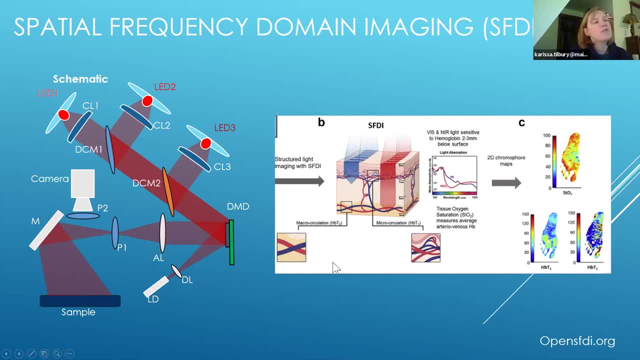 And then I'm going to simply take a picture of that projected light. So over here here's a cartoon version from a paper that is not my work, but I'm following. in this work We have two different wavelengths of light, So we have this blue wavelength and this red wavelength and see that we have like bars being projected onto that tissue. 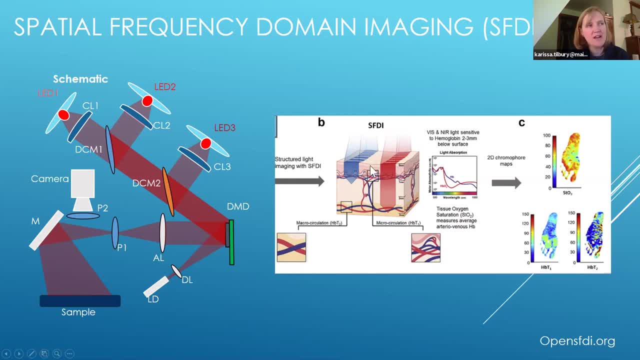 So, just like a barcode, we're going to project a barcode of light onto your skin And, depending on the wavelength and the barcode frequency of light that we're going to project, we're going to sample different volumes of our tissue. So here we're seeing that we're sampling a much shallower version. So this is going to be the capillaries, those purple loops that we saw in the previous slide, versus the red light is going to penetrate deeper and is going to get into this arterial region or the 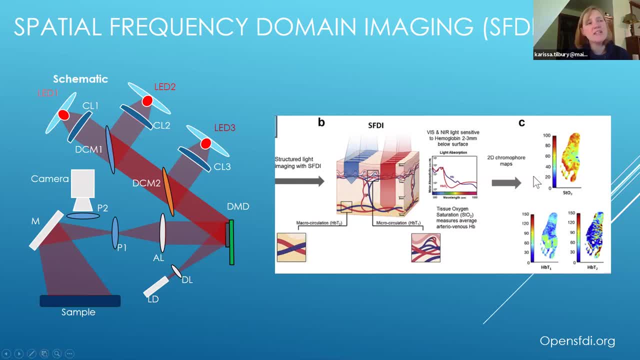 the macular circulation. Okay, so what they did is they did this on a bunch of human patient volunteers and they looked at the oxy and deoxy hemoglobin. So your blood carries oxygen with it. So what the pulse oximeter is measuring is how oxygenated your blood is. So what they're doing here is they're measuring the oxygenated versus the unoxygenated blood at two different layers, So the top and the bottom. So this is going to be T1 and this is T2.. 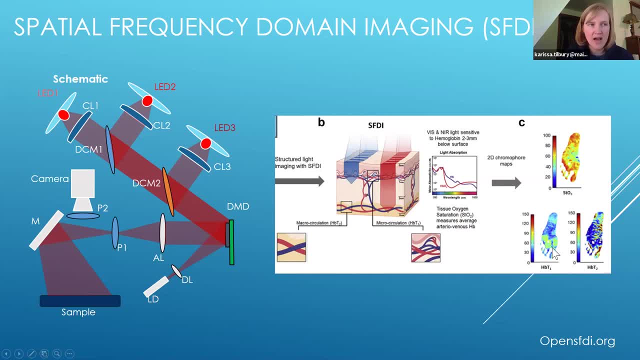 So you can see that the hemoglobin maps, the oxy hemoglobin maps of those two different layers look very different. So that's giving you an indication of how the blood is flowing through your feet to meet the oxygen level. So, going back, circling back to that physiology, 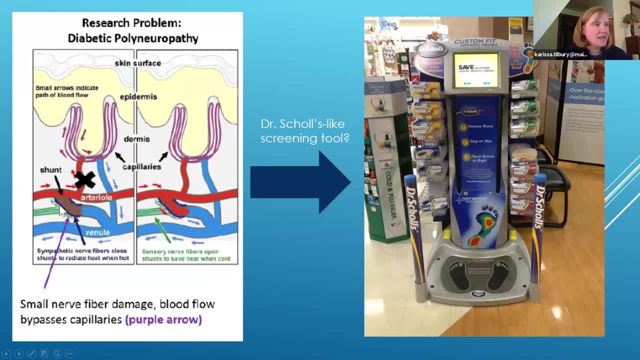 we'll be able to tell, hopefully, whether or not these arterioles are actually pulsating in size and have those nerves intact or not intact, but in a much earlier state than you can respond to if you feel a prick or not a prick on your toe or finger. 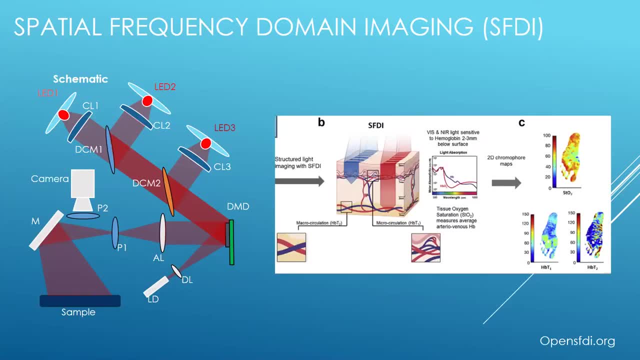 Hi Dr Tilbury, we have a couple of questions For this screen. right here we have the question of what do all those lenses do All these lenses? they are just culminating the light. So if you look at a light bulb in your room, in your house, right, you have this. 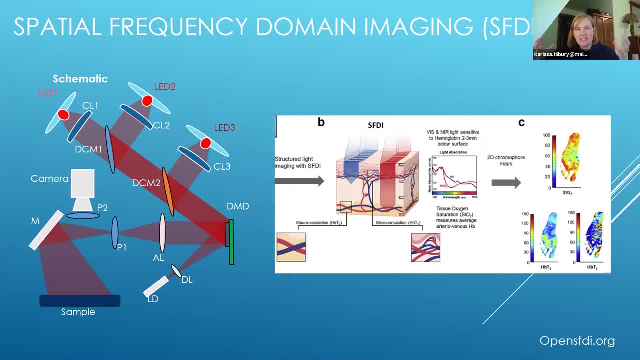 typically piece of glass surrounding it, And what the glass there is meant to do is. it's meant to disperse it and allow the light to get into all the crevices of your room, And in this case, I don't want light to do that. I want it to be focused in on. 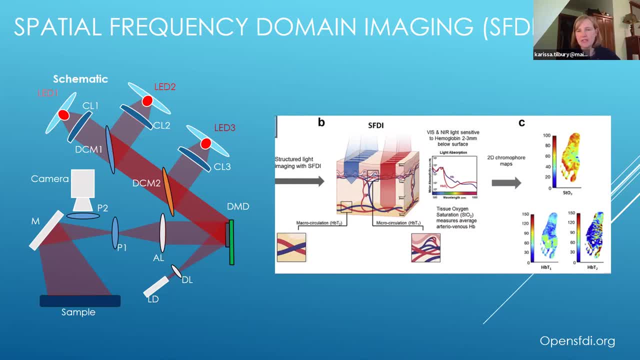 where I want the light to be directed to. So that's what those lenses are doing. Okay, And we've got one other question: What does chromophore mean? Chromophore, Yeah, So a chromophore is a substance that is a tissue absorber. 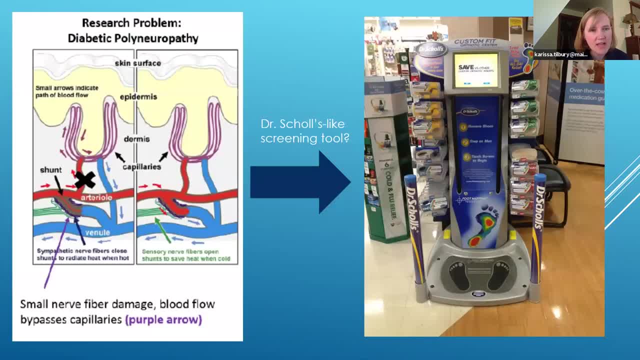 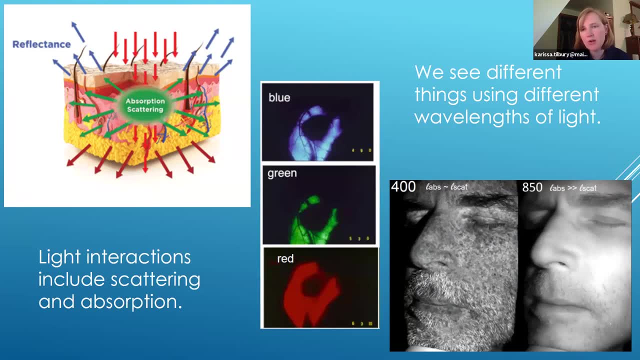 So remember on this slide here, this green absorption or scattering, So chromophore is going to be a chromophore, It's going to be something that is absorbing light, So I'm not going to be able to detect the photons either transmitted through or reflected back out. 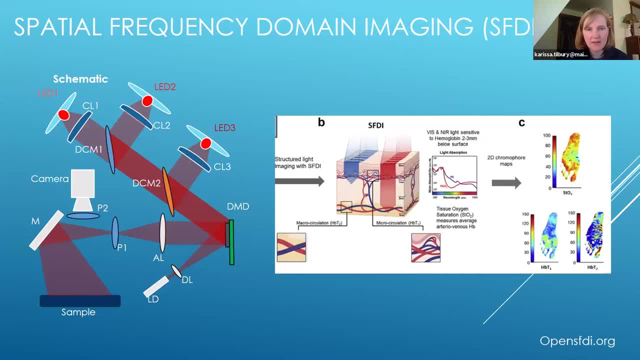 And I should add that oxy- and deoxyhemoglobin. it's sort of really small here. So this is, two chromophores are pretty common are oxy- and deoxyhemoglobin. That's what your pulse oximetry is measuring. 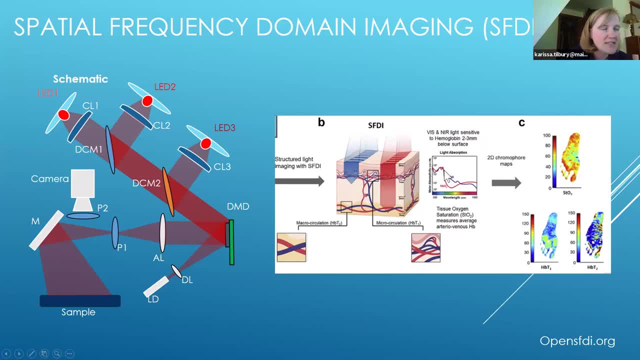 So if you see, in red here you have this oxyhemoglobin map And it's a function of chromophore, It's a function of wavelength, So this is how absorbing it is. So it's very absorbing at blue-like wavelengths And the oxy- deoxyhemoglobin is labeled here in blue, or HP. 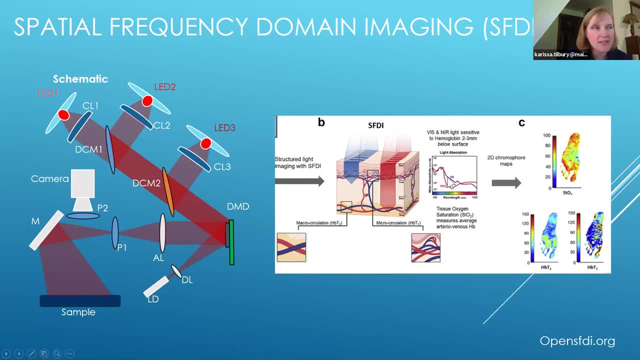 And it has a difference. So, just like in pulse oximetry, you have multiple wavelengths, So you can have a wavelength here and then a wavelength here. So you're going to be able to just think, to differentiate what the absorber is by the ratio. 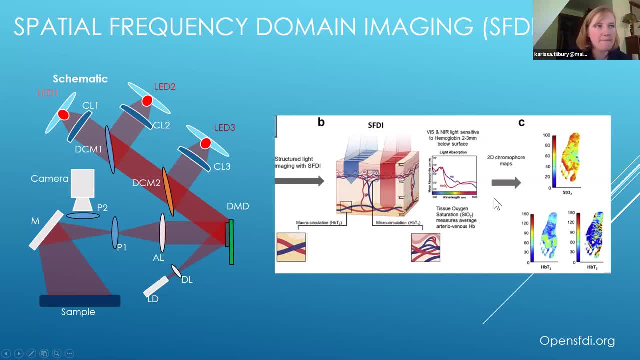 Of that, those values. Any other questions? Nope, that's it for now, All right. All right, So a little bit under the hood, So I can create these beautiful images right, And I can look at differences of micro and macro circulation. 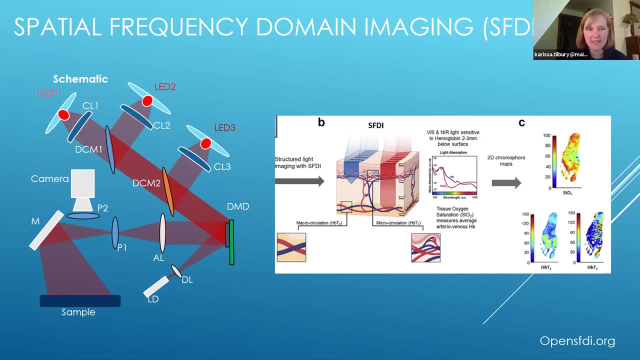 But exactly how do you go about doing it? So I have this image schematic set up. So, also at the bottom of the slide, I have opensfdiorg, which is a website that I'm a part of creating material for, And if you go there, there's step-by-step instructions on how to make your own, very own, spatial frequency domain imaging system. 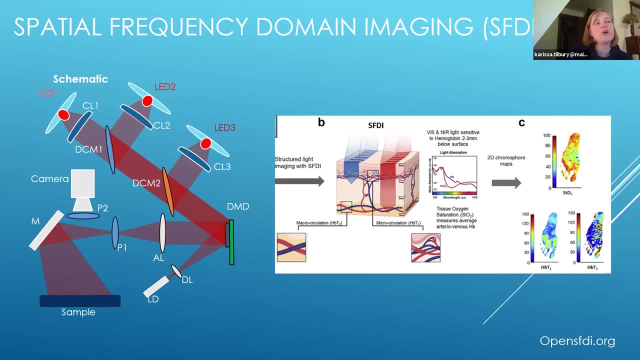 And there's even some pseudocode there in order to look at how you go about processing these images. So I wanted to just take you a little bit further under the hood, just to gather some sort of appreciation of what it takes to get to this point. 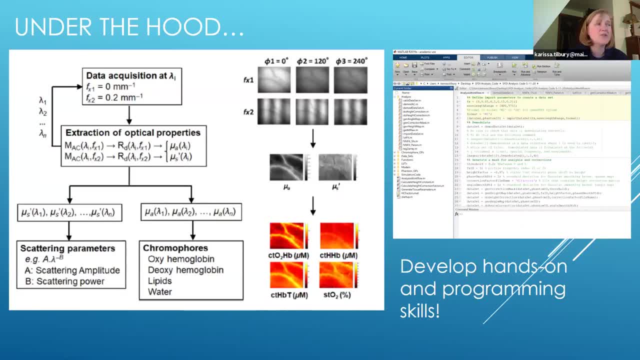 So, after you have the instrument built, you'd have to do, you have to, of course, acquire your data that you're interested in, And so this is a flow chart looking at how you might go about acquiring and then extracting, and there's representative images over here. 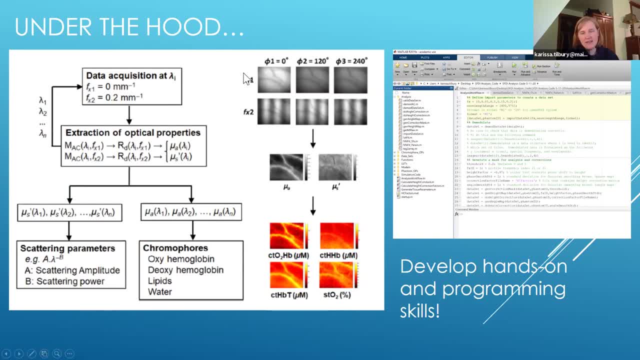 So I have two different frequencies. So I have a DC. So you see, in this top row here we have images that look like uniform light distribution throughout the entire thing, And then I have an AC frequency down here in this FX2.. 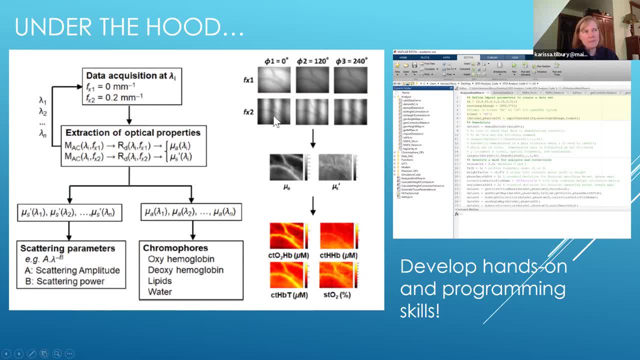 So at this point this is looking like the bars that I'm projecting onto the tissue. So I'm going to take that bar and I'm going to rotate, I'm going to shift it in space or actually in phase here. So I have a sine pattern that's generating these bars. 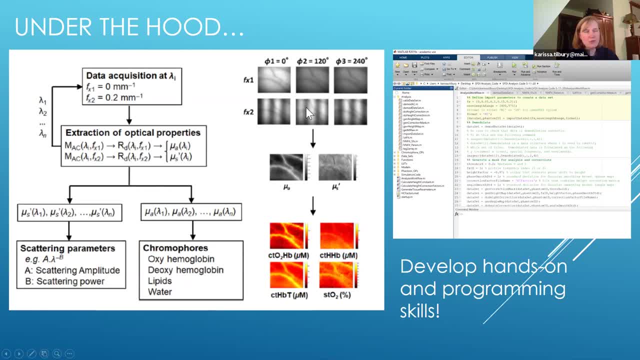 and a sine pattern at zero, And then I'm going to shift it Over it by 120 degrees. I'm going to shift that so you can see that no longer are these bars in the same place, but they're still the same size bars. 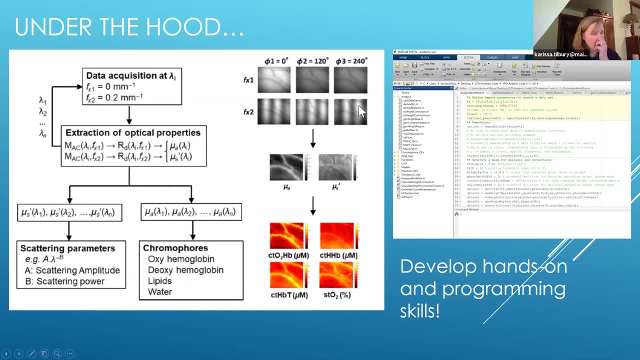 I'm going to shift it once again 240 degrees And then I'm going to go through a process called demodulation, And demodulation is a way in which I'm going to look at all these. I'm going to take all these images and combine them all into a single image and get rid of any phase information. 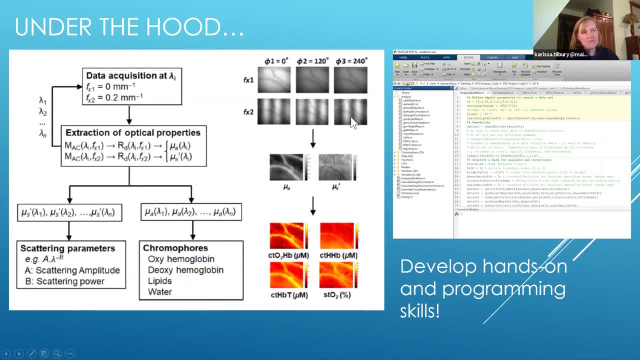 So I'm going to collapse these down, And when I collapse these down, I'll effectively have a planar or an AC image that looks just like this, And the reason that this is important is because anything that's going to be the same across all those images. 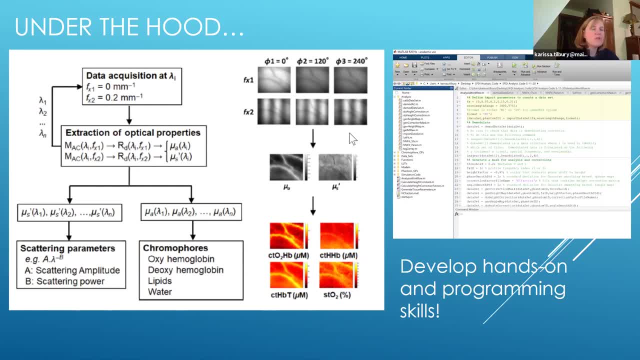 I'm going to get rid of, I'm not going to care about that anymore. So from that then I am into a space called diffuse reflectance space And I'm going to get images that, from that space, I can look at and understand how absorbing and how scattering. 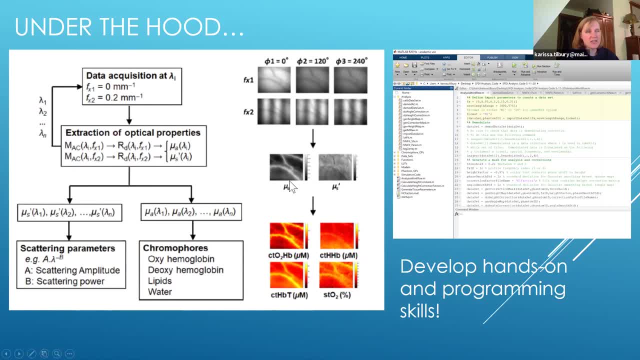 are those two particular tissues. So from these six images I can get these two images, And then from these two images I can look at particular tissue chromophores. So oxy and deoxy hemoglobin are shown here, So I have total oxy hemoglobin. 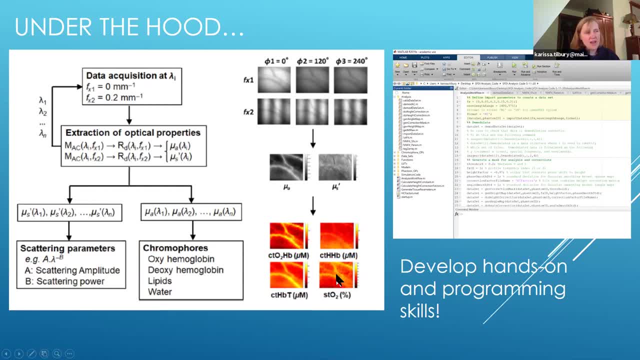 total hemoglobin, total deoxy hemoglobin and then percent saturated O2, which are just derivatives of each other, So they're addition and subtraction of them. So all four of these images are coming from this particular UAA image, right here. 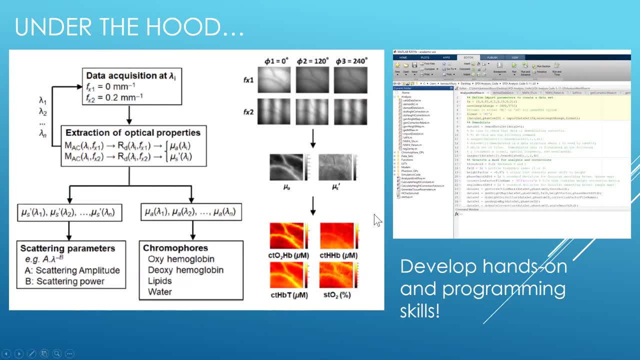 We did have a quick question: Why do you use bars? I? the reason we use bars is it's just a really easy, simplistic pattern that we can use to project, So you could use any shape that you want, but you're going to make the math a lot more complex and there's not really an upside for it. 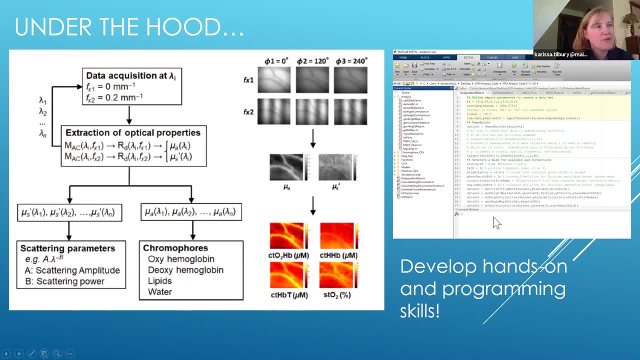 So what I did over here is I took this flow chart and I showed you the front end screen of what our simulation or, I'm sorry, our analysis code looks like. We also have some of this for simulations on the other side, So it has multiple parts. 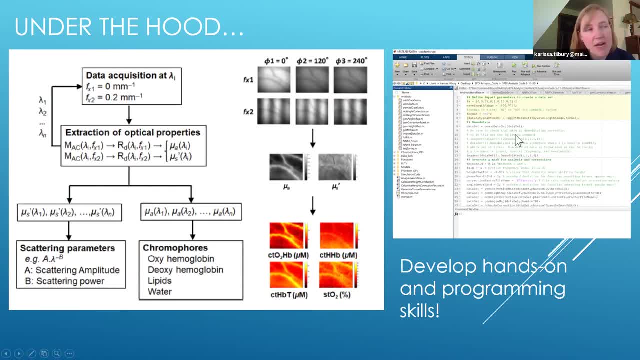 So this is just sort of a loading in part up here. This is our demodulation part Here. So it's going to take these images and create a single image, And then we can create masks, We can do other things, and it's going to go down. 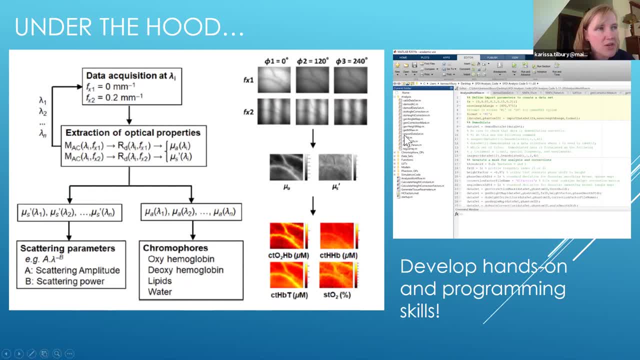 So over here you can see, there's several functions that we're going to use. They're all being called from this main program to do all this work, to eventually get us these images so that we can quantify what in fact is happening in that. 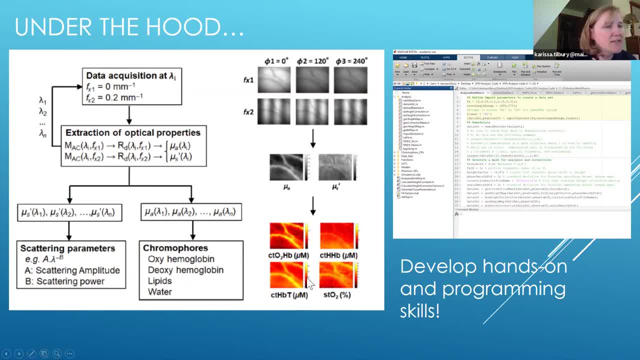 So it's complex. There's lots of hands-on skills, There's lots of developing program skills and communicating with other people. So you don't have to be awesome At all of these, these skills, but you need to be willing and curious to learn about, about these things. 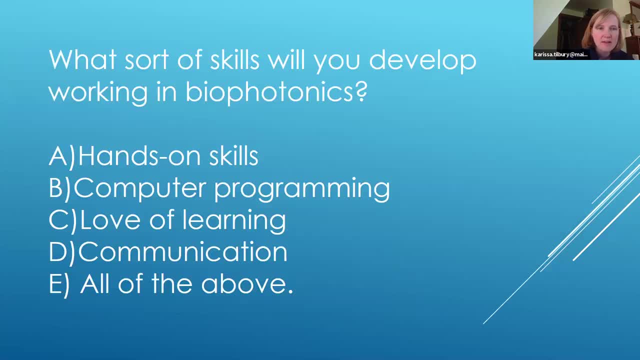 So that leads me to my last poll question of the day, which is: what sort of skills will you develop working in biophotonics? We are almost there. We've got 90% of our participants have voted. We'll give them just a few more seconds. 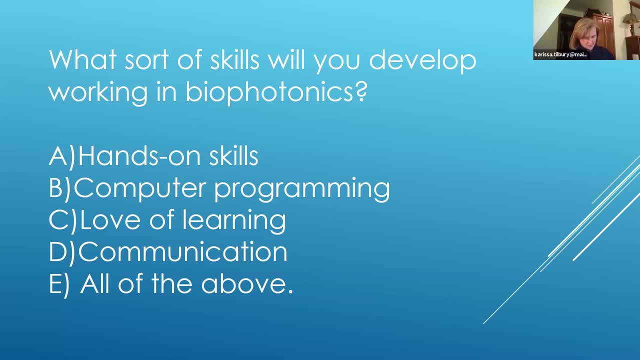 And share the results. All right, All of the above 80%. for those of you who said hands-on skills and computer programming, you are also correct, But I just wanted to have have all of the above, And you notice that I also put in a love of learning, because we're never perfect at any of these things. as you go along. 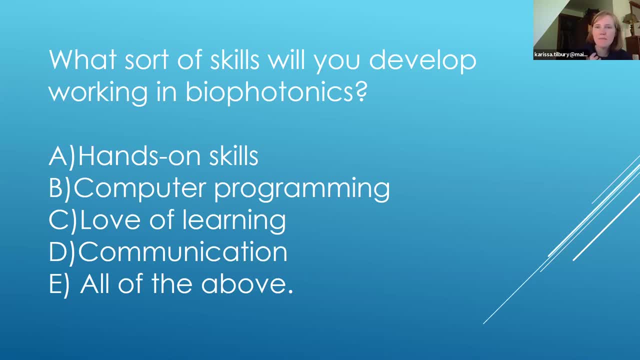 So in the next couple slides I thought I'd show you. First of all I thought I'd show you sort of some students that I have in my own lab that both started with me as freshmen And now one's entering their junior year and one just graduated and kind of what their pathways look like. 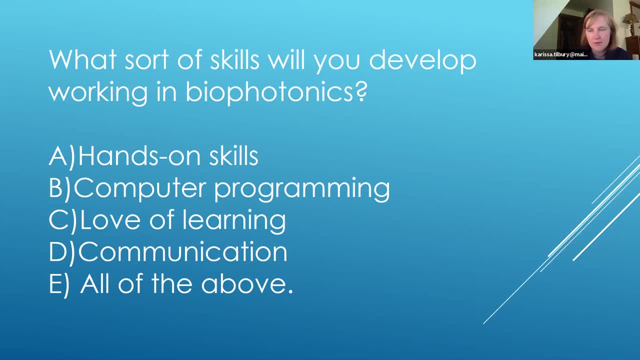 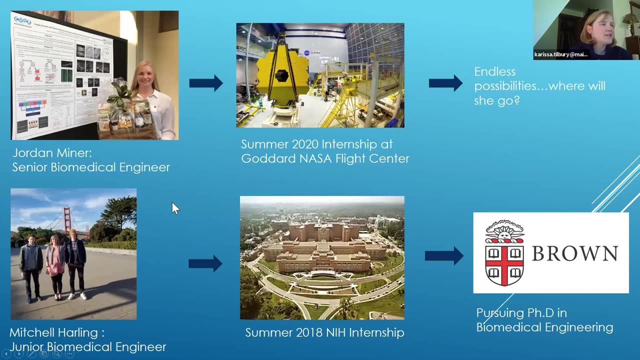 And then I'll enter what my pathway look like and then I'll open up to questions and answers that you might have. All right, so these are the two students that I've had in my lab since their freshman year. So the top, her name is Jordan Miner and she's an incoming senior in biomedical engineering. 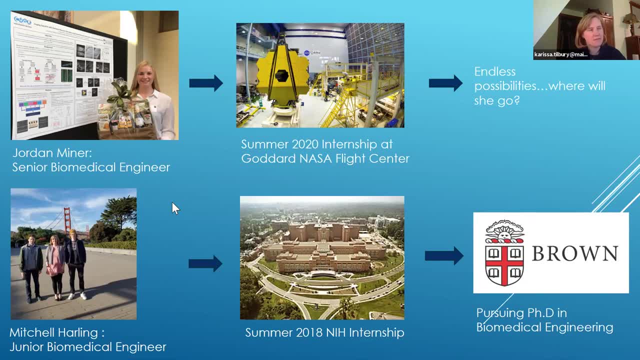 Now you don't have to major in biomedical engineering to be interested in biophotonics, but it is a pretty good major to choose. So she's pictured up here. She won a poster presentation at the Northeast Biomedical Engineering Symposium, which was really an awesome thing. 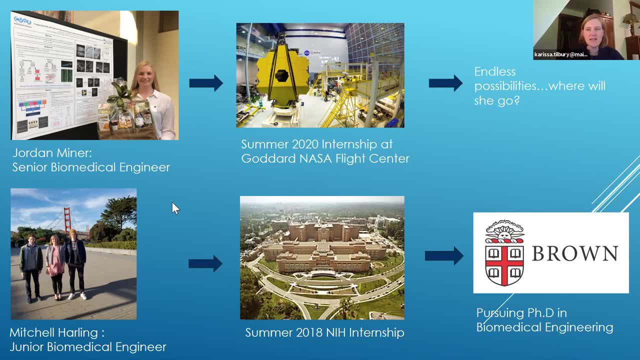 Feet, because this conference is mostly attended by postdocs. So postdocs is a thing. They probably are not aware of what they are. So postdocs are people that already have gotten their PhDs and they're working in labs and receiving more training so that one day, 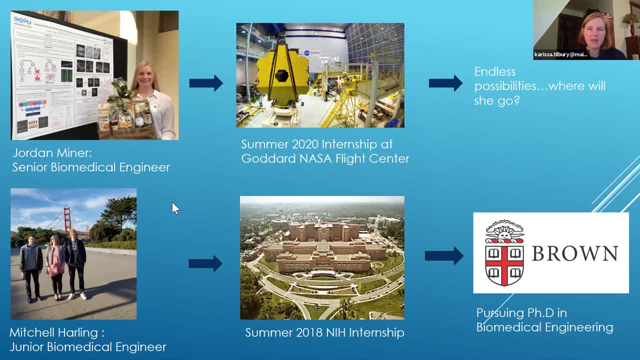 hopefully they might become professors or work in industry as well. So she won that in a field of lots and lots of postdocs. So that was really quite impressive, And in fact she was competing against postdocs at institutions like MIT and Harvard and Boston University. 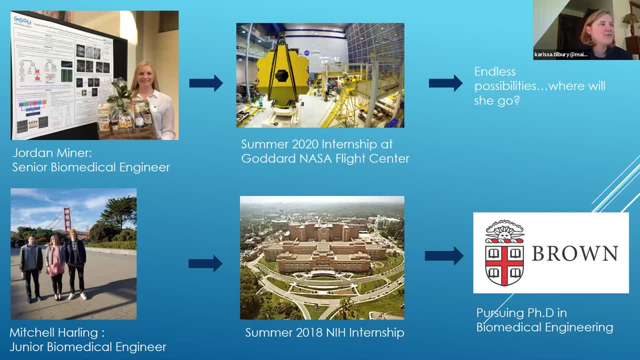 And funny and real true story. She- I was not there at this conference And when she returned she told me that a professor from MIT thought that she was a third-year postdoc and was floored when she's told him that no. 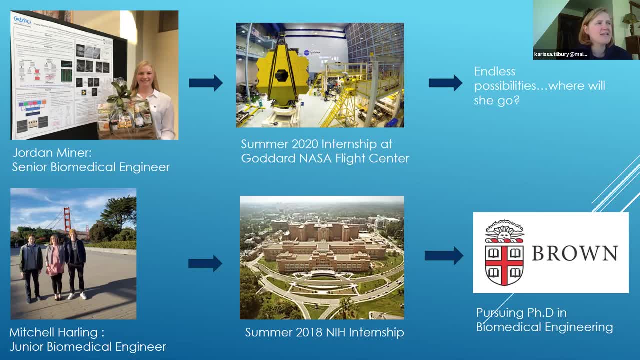 she was a third-year undergrad. He was also asking how we got such good images that we are seeing on her poster. So this is a different optical technique that I use in my lab And we're looking at myosin in terms of health and that approach and understanding muscular dystrophy. 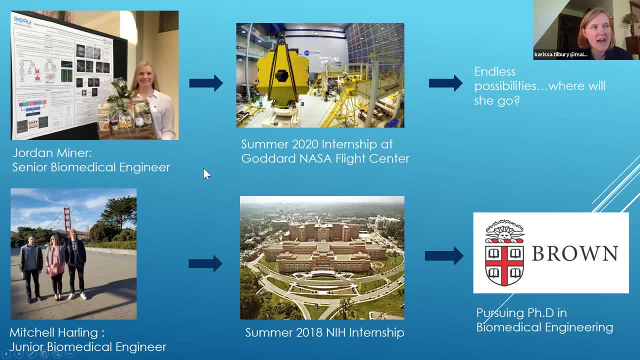 So I'm happy to say that she is awesome And she is now doing a virtual summer 2020 internship at the Goddard NASA Space Flight Center, So hopefully she gets to go down there and visit before the summer is done And then she'll be coming back to UMaine campus and continue her work on the zebrafish project. 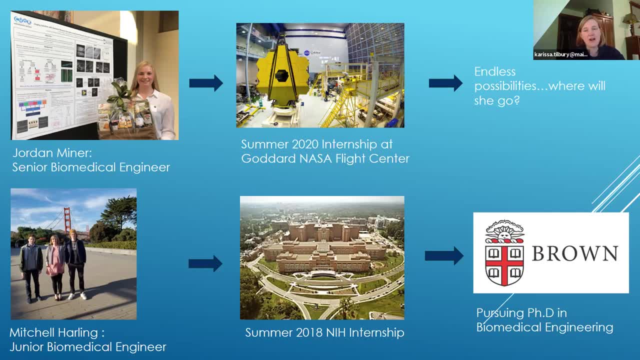 And you know I'm really excited to see where she goes. Possibilities are endless. I think she's going to learn even more in terms of what's out there after the summer internship at NASA. Another story: Mitchell Harling. he is. 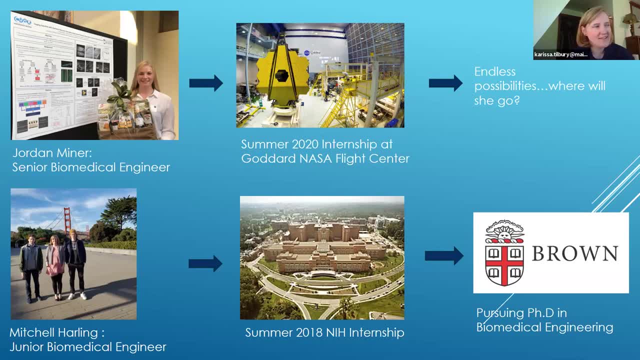 he is not a junior in biomedical engineering. He just graduated. He's a 2020 alum. So he went out with me and a grad student, Wyatt Austin- picture on my left- and presented as an undergrad at the largest biomedical optics. 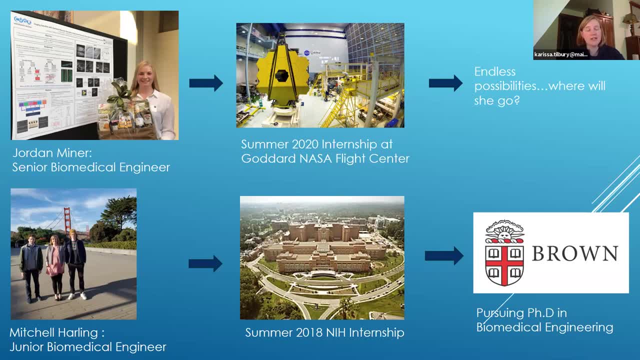 conference in the world. It's called SPIE, Photonics West, And after they presented we had a little bit of a fun day and we went and saw the Golden Gate Bridge And it was, it was great. So what other opportunities has he had? 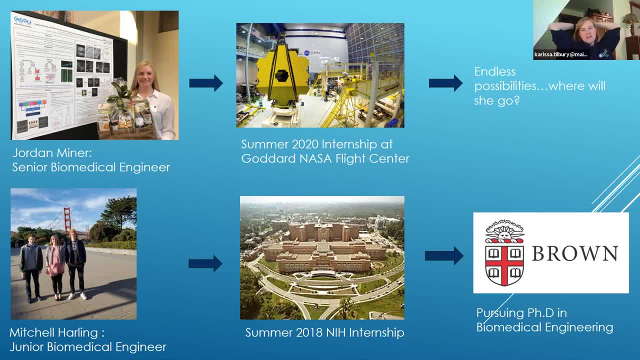 So in the summer of 2018, he was an NIH National Institutes of Health intern and he got to work in this research campus down by Washington DC area. And where is he off to? Well, he's off to pursuing a PhD. 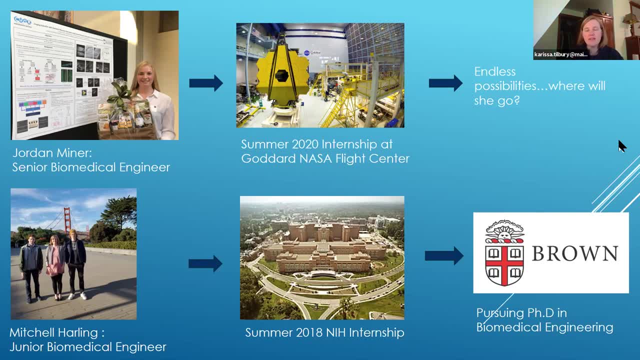 in biomedical engineering, where he's going to continue the work that he started in the biophotonics community as a PhD student in the probe lab at Brown University. So it's really, really, really exciting And I'm thrilled to see where they end up. 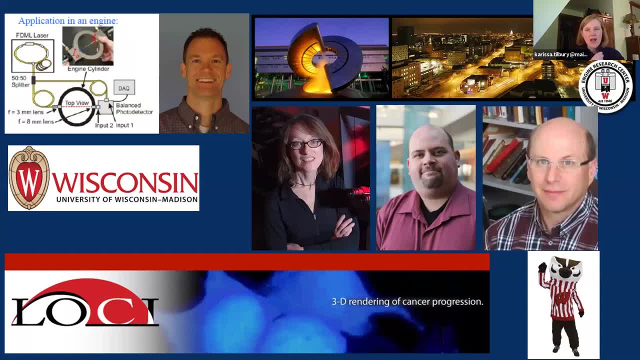 All right, so a little bit more about my pathway. So I grew up in rural Wisconsin. I had no idea what engineering was until I was applying to college. I thought I wanted to go to medical school And I was sitting in this seminar and I learned about biomedical engineering. 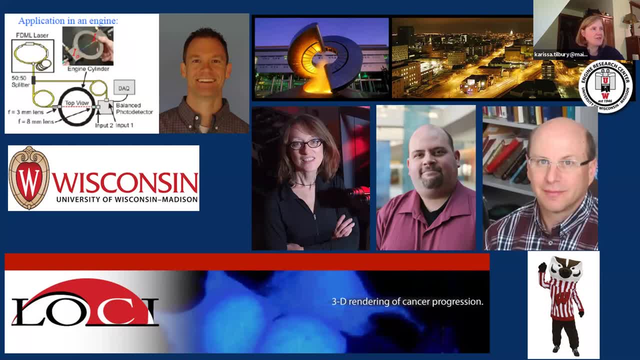 I was like, wow, that's so cool. I had no idea that that was actually a major, because I was kind of doing the classic debate: Do I do biology, Do I do biochemistry? You know, I really didn't know. 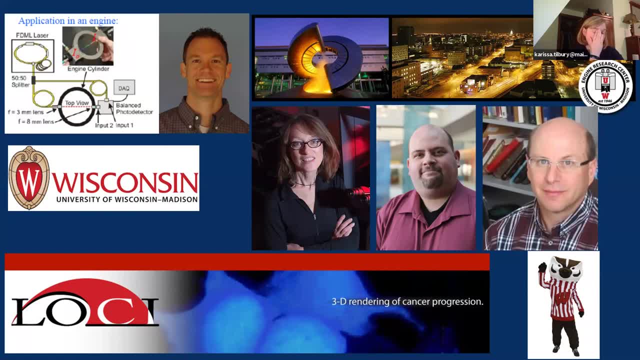 So I entered. I was a badger Really excited by that And I dreamed about being a badger The entire life. So when I got accepted, that was exciting. I, as a freshman, I was had a job on campus as a janitor. 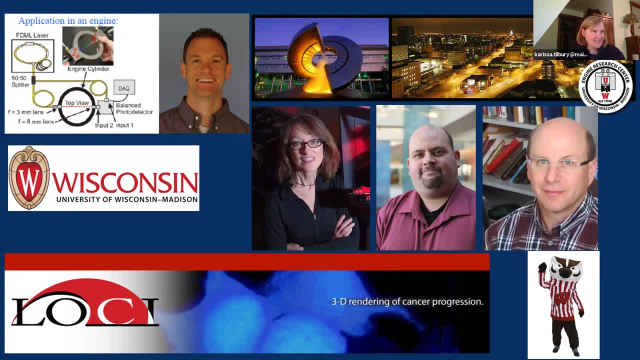 and I really didn't want to be a janitor because it really sucks. So I found a different job and that led me to the first kind of purview into biomedical optics, but not in a healthcare way at all, So my first entrance into biomedical optics. 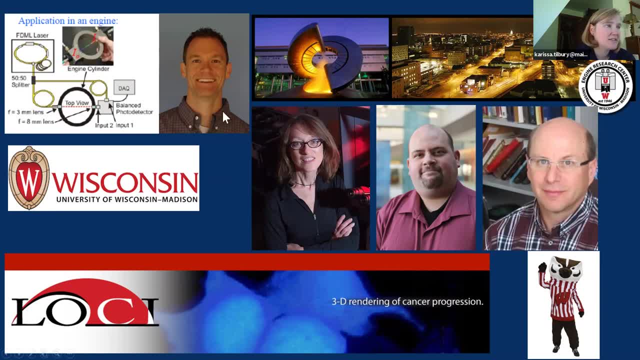 or optics in general, was with this person here, So his he was my undergraduate research advisor. His name is Scott Sanders and he's a mechanical engineering professor, and he uses light to understand what's going on in the combustion process inside car engines. 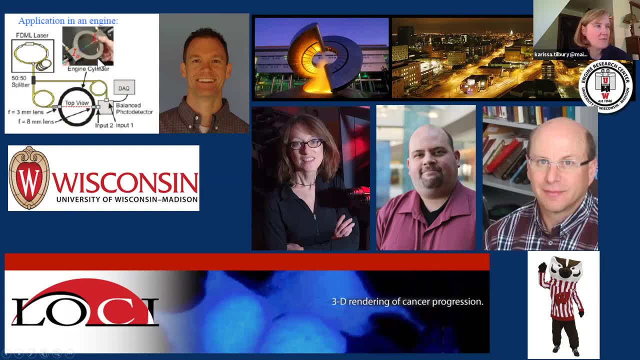 So you know, really the farthest thing from my thought process. I wanted to do things that were related to health, not and not car engines, but it was really cool. So basically, he, you know, used a light. 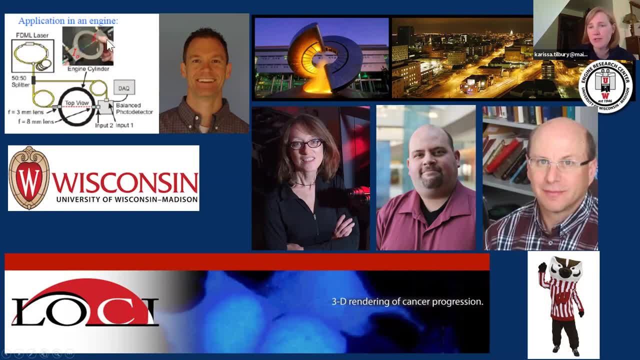 used different wavelengths and measured the absorption coefficients across the the cylinder range in that approach. So through meeting him, I stuck with him all four years as undergraduate researcher. He introduced me to Kevin El-Siguri, who also introduced me to Patty Keeley. 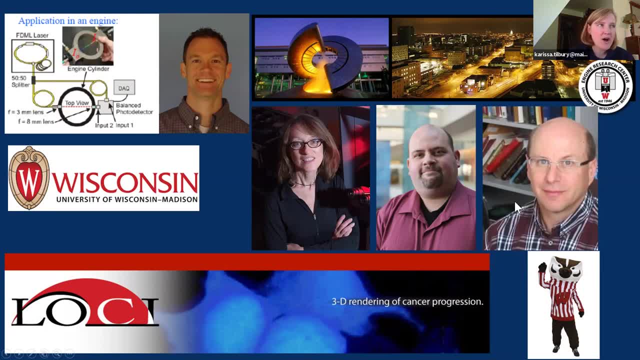 and ultimately my PhD advisor, Paula Campanula. So I continued on at the University of Wisconsin at Madison for both undergrad and graduate careers. So this was our engineering hall building and it had this really cool water fountain that we could control. 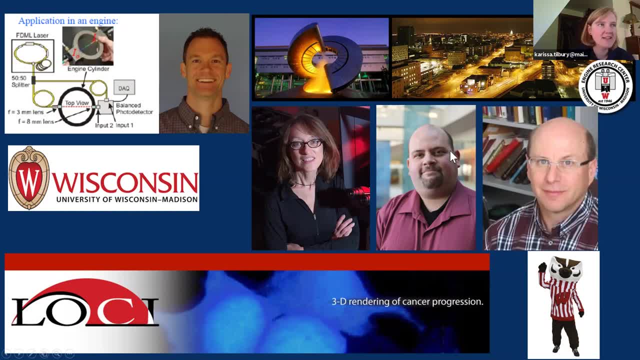 Students could control the lights and how the water was coming out of it, And this is what the campus looks like at night: Highly highly photoshopped to have that blur. And as part of my studies throughout all these groups, I was a participant. 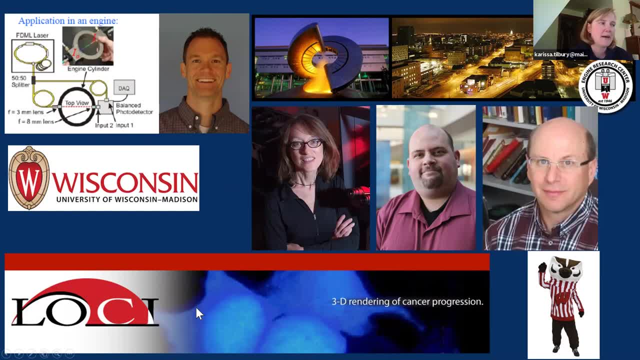 active participant in a lab called LOCI, which stands for the Laboratory of Optical Computer and Instrumentation, And it was this really unique place. It was a place in which biologists, physicists, computer scientists, biomedical engineers, electrical engineers all came together and created instrumentation. 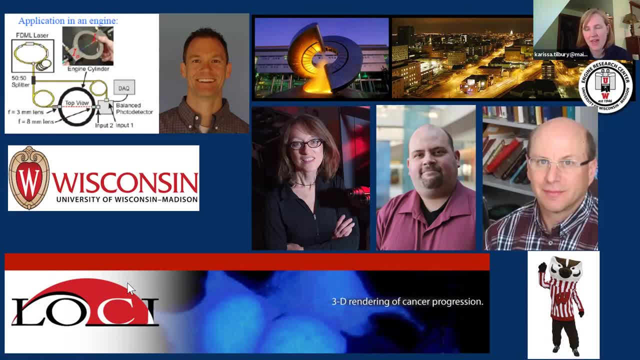 and then applied it to biology and health questions. So it was really the brainchild of Kevin El-Siguri, and he was supported by lots of other PIs, both of which are pictured, and I interacted with a lot, So Patty Keeley and Paul Campanula were both active participants. 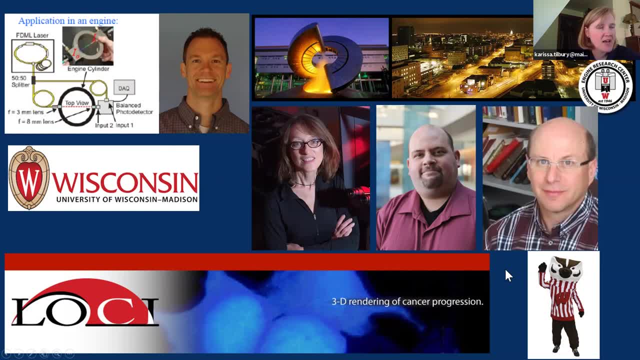 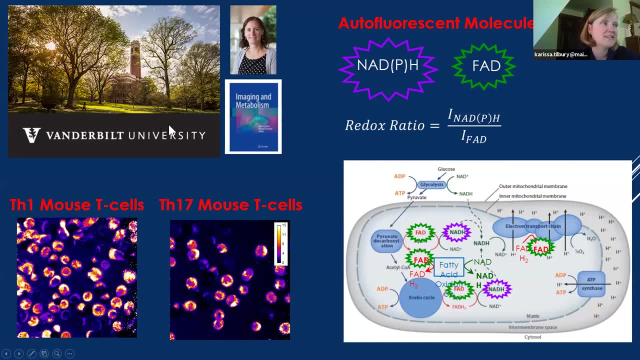 And so after I got my PhD in 2015,, I did a short postdoc at Vanderbilt University in Nashville, Tennessee. This is a picture of the beautiful campus. It's very green in comparison. So I continued on this optical path. 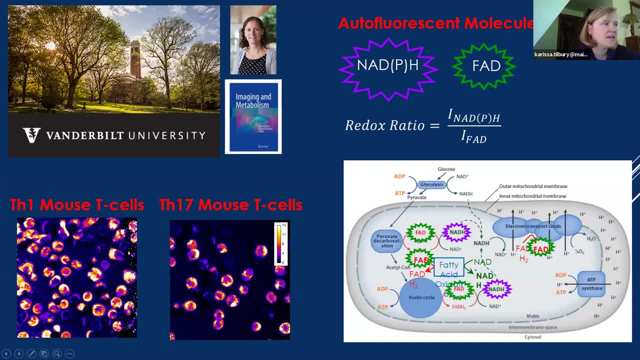 So what you're seeing here is T cells from mice, So two different types of T cells. So we have TH1s and TH17s And what we're seeing in terms of their contrast here is the ratio of two enzymes, NADPH and FAD. 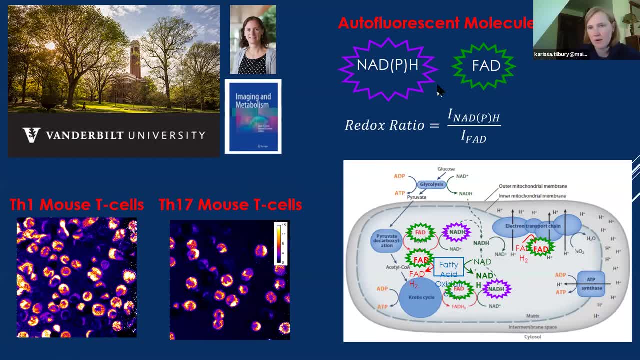 which are autofluorescent, meaning that I can see their, they absorb, And then, after they absorb, they emit some other color of light And I can collect the other color of light after I excite them, And they do that without adding anything to them. 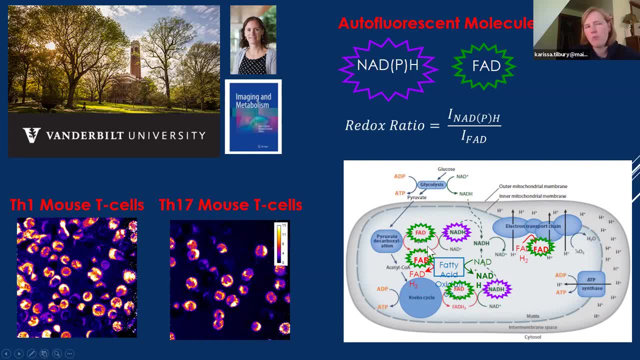 So I can take that ratio and I can tell you sort of what sort of pathways is a cell using in terms of metabolic process And why that's particularly important is we can understand cancer. that way We can understand differentiation of stem cells. 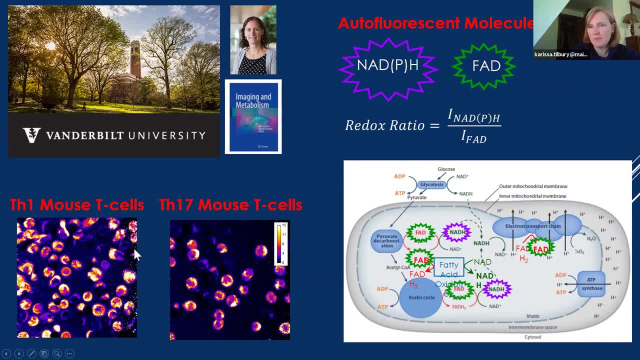 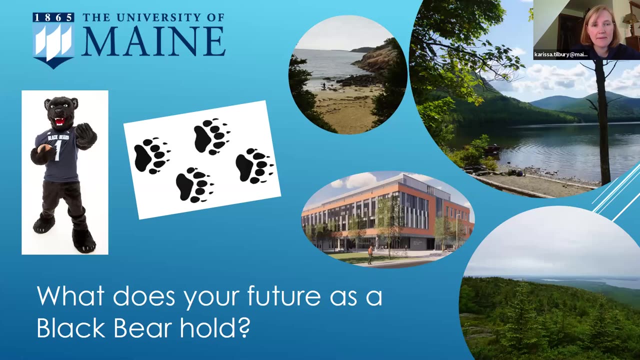 And we can also understand how, what type of T cell we have, which is becoming more and more important in terms of understanding immune cell function, both in terms of viruses, bacterial infections, cancer, et cetera. So then, the last step was really here as an assistant professor, and I traded in my Bucky. 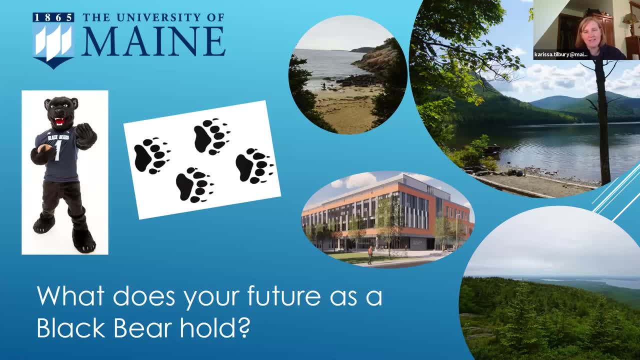 Badger shirts, which I still might have a few, but they're starting to dwindle into black bear shirts and became bananas and, you know, started out my career here as an assistant professor. So I invite you to consider what is your future hold as a black bear. 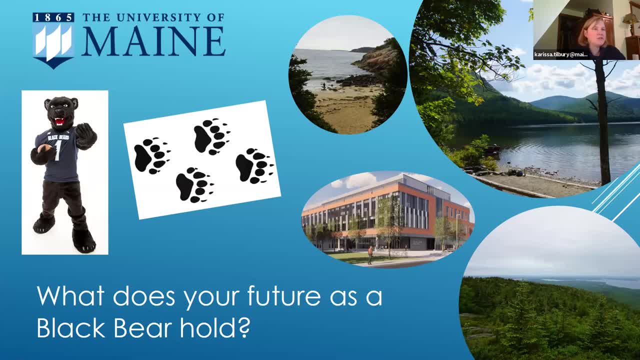 So we live in a gorgeous state. These are pictures from Baxter State Park and then Acadia, And I also just wanted to say: put a plug in if you did. if you did not know, there is a brand new building that's going to be aligned in about two years. 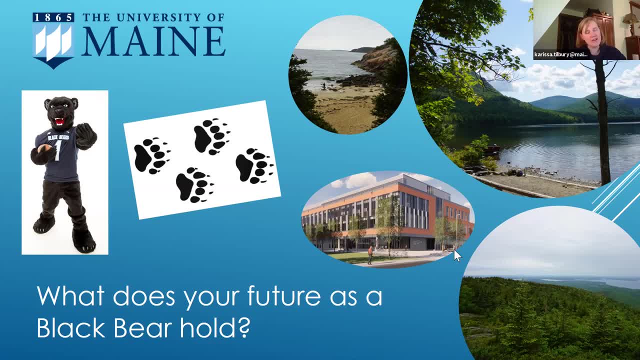 And biomedical engineering is going to get the entire third floor. We have brand new research labs and brand new teaching spaces And there's going to be a brand new biomedical optics suite in there, So it's just going to be really great times to consider being a black bear. 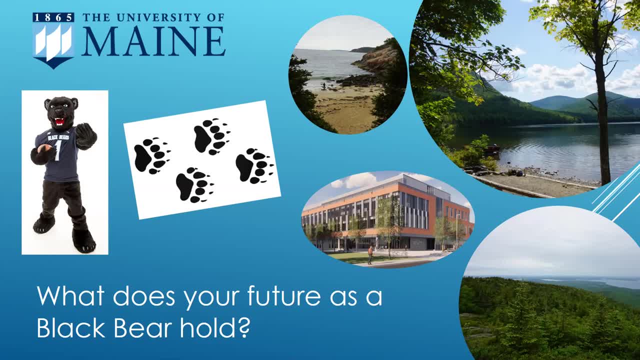 And we did have a question come up when you were talking about the seminar where you learned about the field you ended up going into. How did you find out about that seminar? Yeah, so that seminar was. I was applying for a program that allowed you to apply directly from high school into college. 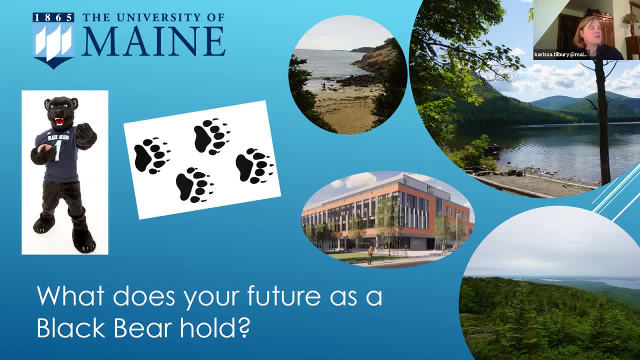 And then, provided that you kept a particular grade point average, etc. Through college you were automatically accepted into the University of Wisconsin Medical School. So it wasn't until I was In that workshop to understand how to successfully apply which I did not successfully apply to. 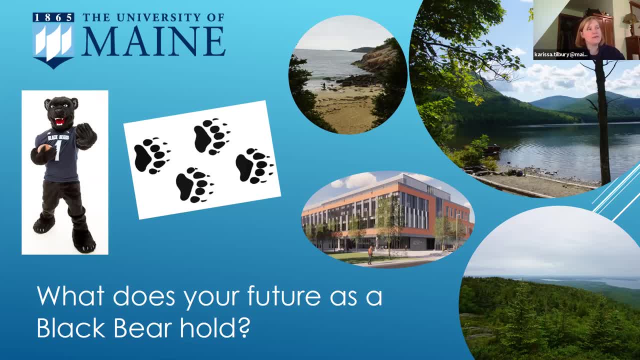 I did not get in, But that's where I learned about that- that entire major program. So, Carissa, if you were sitting here as a high school student, how do you think you would find out about types of opportunities like that at UMaine? 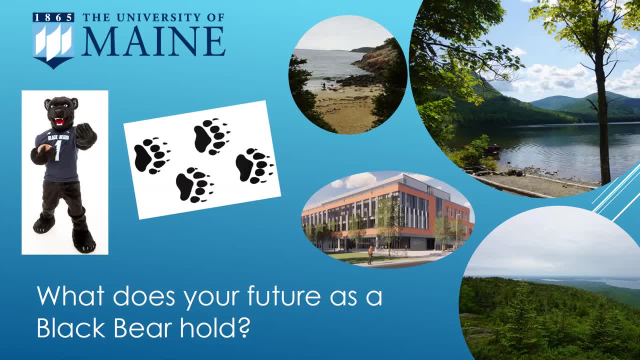 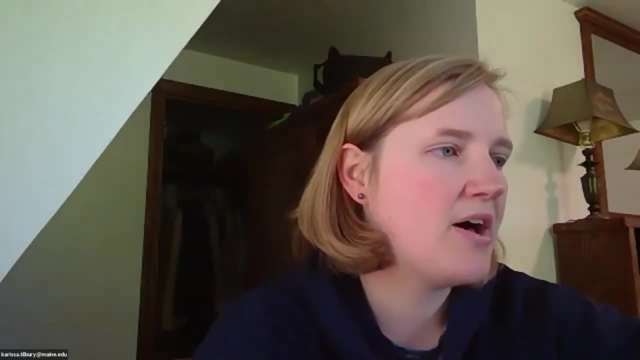 I know our UMaine admissions folks have a lot to offer. Yes, So I would say admission is great. You can also reach out to individual faculty members. Like I've hosted high school students doing research through Upscore, We also. 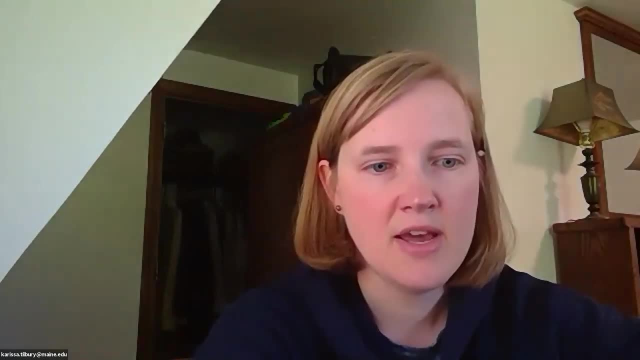 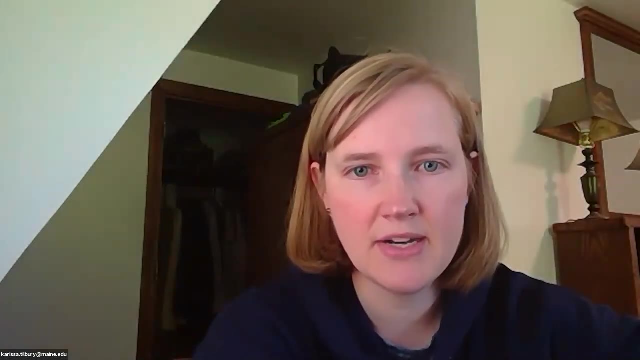 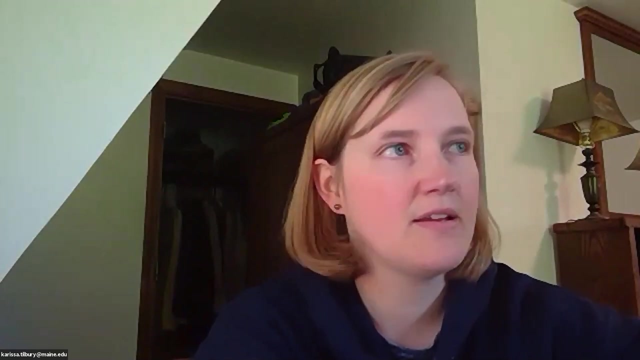 I want to show you another thing. There is an upcoming camp- This one's for middle schoolers, but there's also a program called Consider Engineering. Okay, you're not seeing my screen? I don't think. No, we're not. 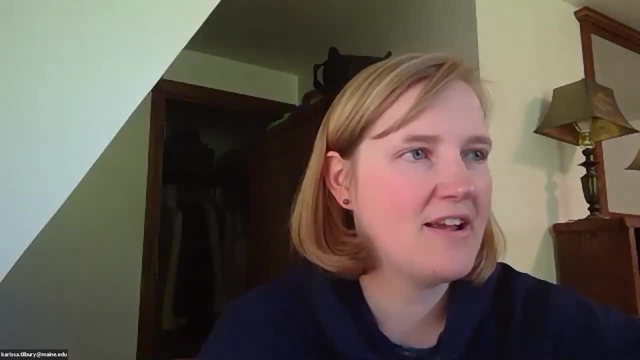 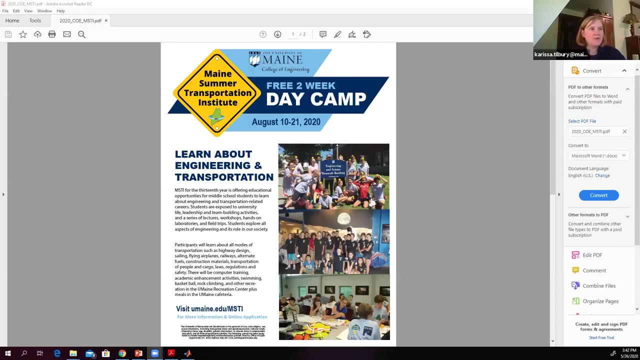 Okay, I'm working on getting it back. Okay, All right, I think I have it. So there's Consider Engineering for high school students And if you're younger than high school- which some of you might be, there is a Maine Summer Transportation Institute camp this summer that is still accepting applications. 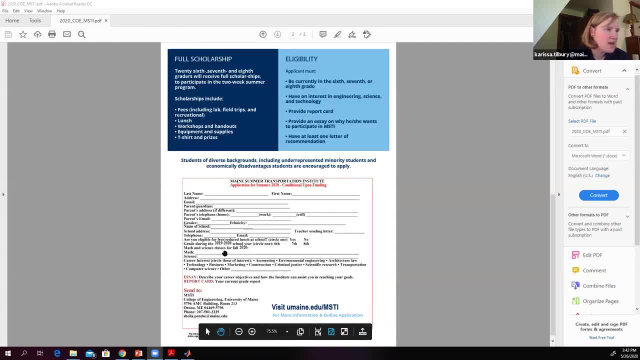 So I am sharing this Flyer with you And if you have more questions, you could email SheilaPenzi at Maineedu and I can supply you that email address in the comments if you'd like. So those are two things that I would say are possible. I have hosted students for research stints during the academic year too. Obviously, it's a lot harder if you're not living close to the campus, but I know one of them was a Maine Math and Science Alliance school and she had a longer J-term. 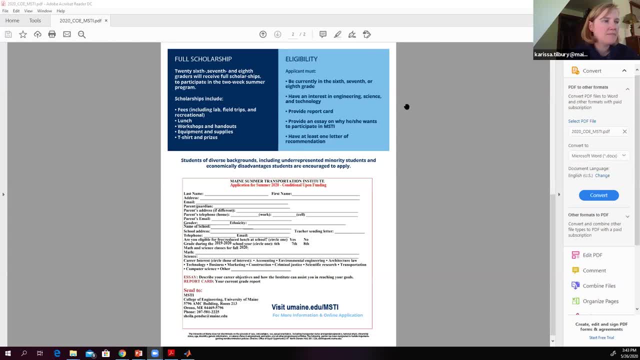 So there's that possibility of doing it in that approach as well outside of summers. I do want to add that through our Maine 4-H program we often do arrange tours and work with the College of Engineering at the University of Maine closely to at least get kids onto the campus. 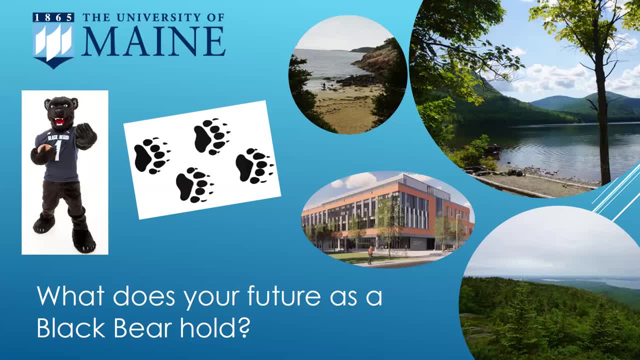 And have them meet some of the faculty. So the College of Engineering at the University of Maine is very welcoming to having middle school and high school age visitors as well. Right now we can't due to the COVID situation, but hopefully we'll be able to bring more people to campus again soon. 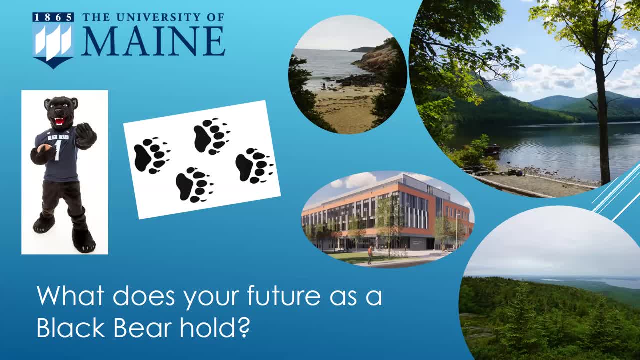 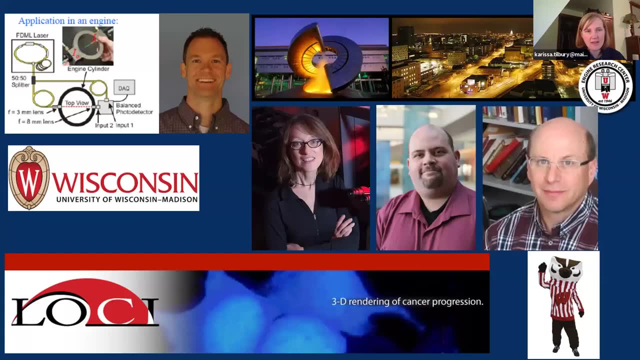 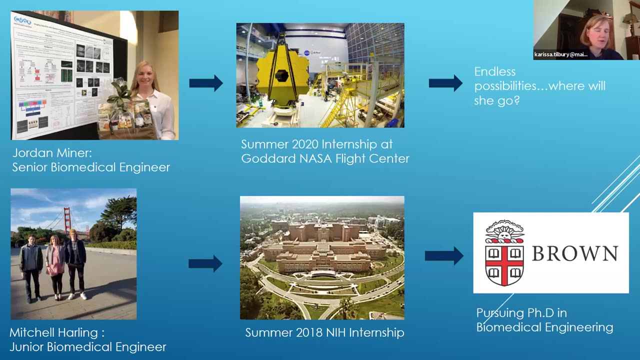 And we did have a question. just come in: Do you work with students at UMaine? I do So. the reason I showed I showcase on this slide. I work with both graduate and undergraduate students and I actually really like working with freshmen right out of the gate. 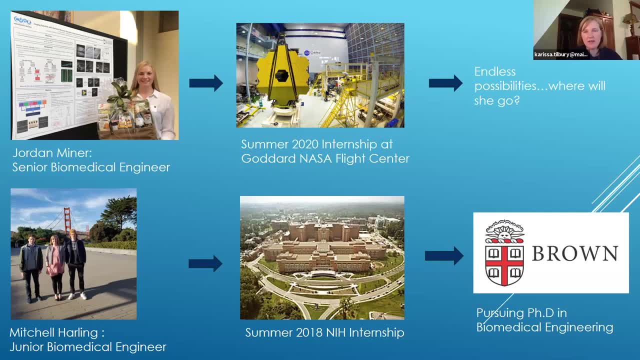 Both of these students I worked with as freshmen, and one's entering their senior year and one just graduated. So these are two examples of two undergrads that I've worked with. When would be an appropriate time to reach out to a faculty member? 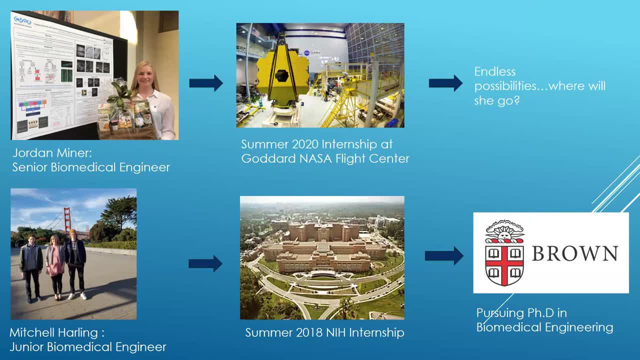 If you were interested in working with them, Would it be after you've graduated from high school? Would it be once you've arrived at UMaine? Okay, you're talking about incoming students, because I was like incoming students. I'm sorry. 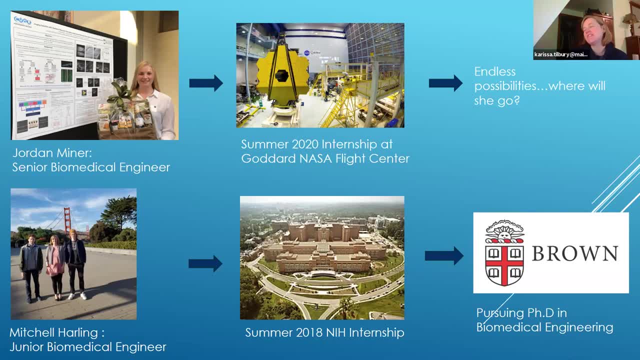 Incoming students, because I was like: okay, because there's high school students, there's incoming students. So, in terms of incoming students, I would say like, go ahead and contact us right away after, right after you get accepted. There's nothing stopping you from interacting with us already. 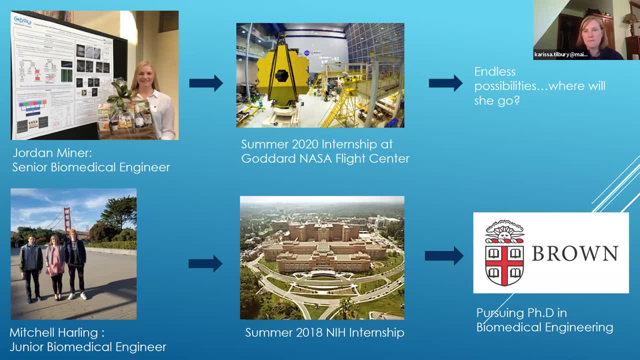 We like interacting with you immediately. I know you will there like in the fall, So we have like, if you're a biomedical engineering student, we have a class that we all come in and actually show what our research areas are to you. So that's one opportunity that you can see the widespread aspects of it. 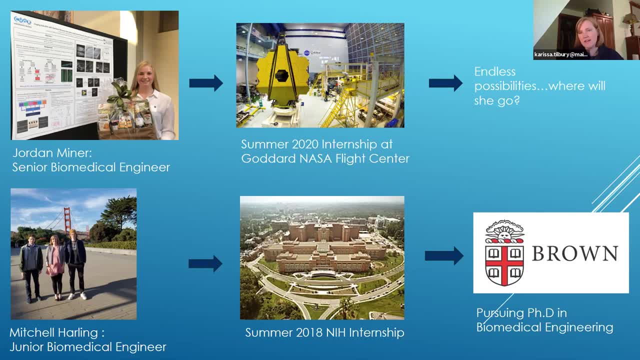 And then maybe you wait until after that If you want, if you want to play on the side of safety. Otherwise, you know you can just email us and we'll get back to you and tell you what we do. Just a reminder. 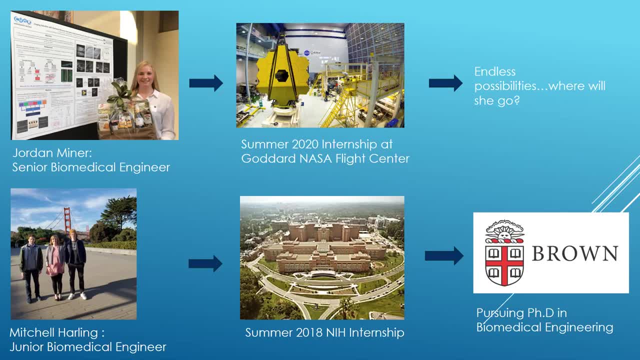 if you have any questions, you can type them right into the Q&A box. We'll give people just another minute or so to think of those questions. I can also say so. this is super exciting, but Mitchell Harleen on this slide. 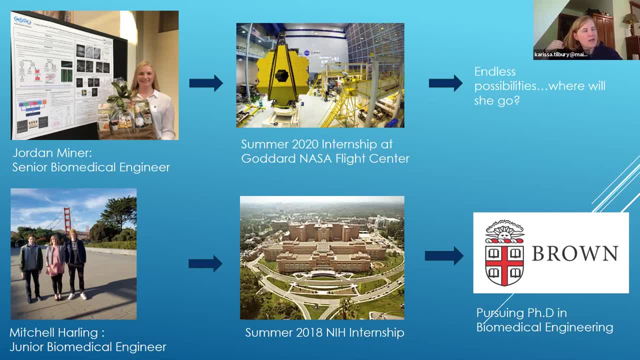 he just got a $4,000 scholarship from SPIE Photonics West. He's one of 78 students in the entire world to get the scholarship this year, And so what he's saying is that, you know, this is a skill that I'm naturally very inspired by. 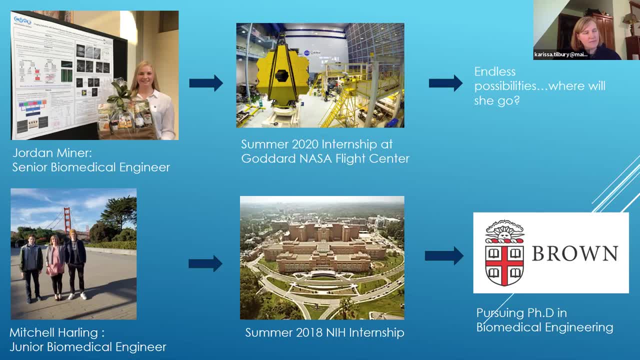 And he's also said I've given some workshop skills. It's still very different than what it was when I was here. I've done a lot of project speaking and we're still doing this initenally and we're still working with the students. 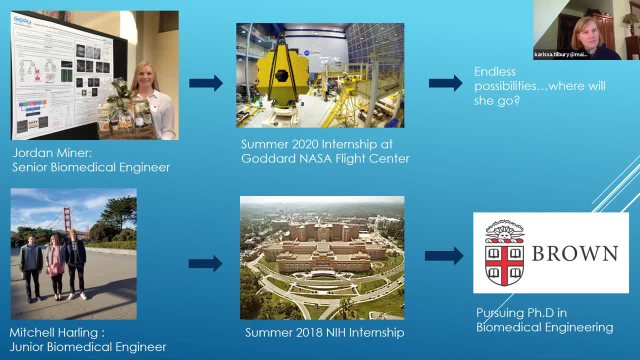 So it's really. it's so much in the last year of my life and I don't think that I've ever felt suspicious of them, because I know that it's a huge thing. It feels like you've answered everyone's questions as we went along. 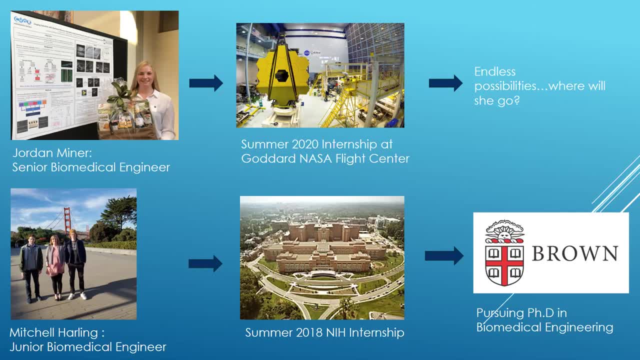 Jesse, are you seeing any more coming in? No, we are all clear on this. And Awesome. Dr Tilbury, I really want to thank you for coming out today. This was awesome. This was probably the most high-tech talk we've had, too, and it's nice to highlight engineering We have. 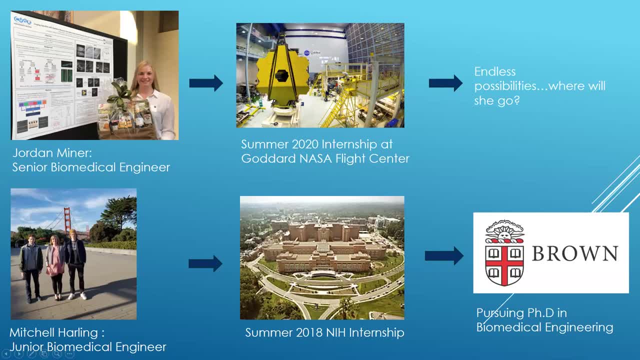 not really talked about engineering before today. I'm going to launch a quick evaluation poll for those of you who are our participants. I'd appreciate your impression of our session, and we are scheduling two more of these at this point Next week. Dr Caitlin Howell is going to 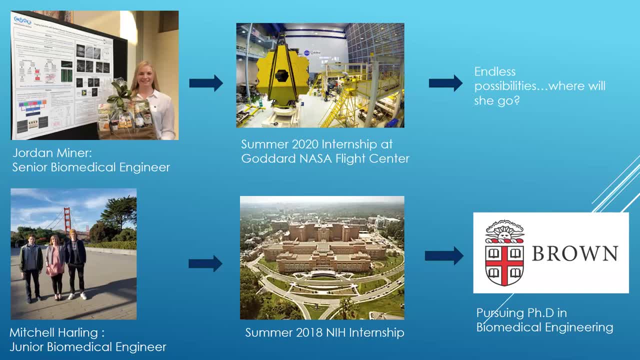 join us to talk about engineering inspired by nature, and the following week we have Dr Tora Johnson, who's going to talk about natural disasters and mapping. so we're pretty excited about those. That's going to be it for our spring quarantine virtual science cafes. We're wrapping.